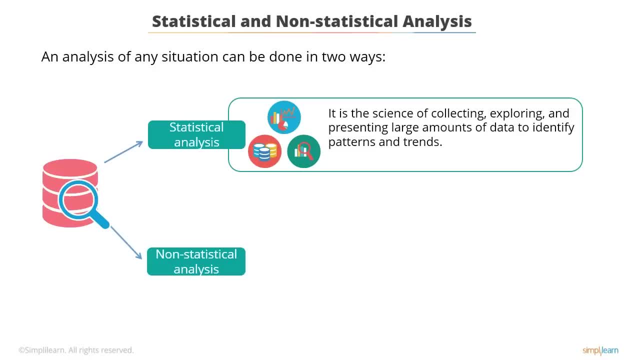 amounts of data to identify the patterns and trends. Statistical analysis is the science of collecting data. Statistical analysis is also called quantitative analysis. Non-statistical analysis provides generic information and includes text, sound still images and moving images. Non-statistical analysis is also called qualitative analysis, Although both 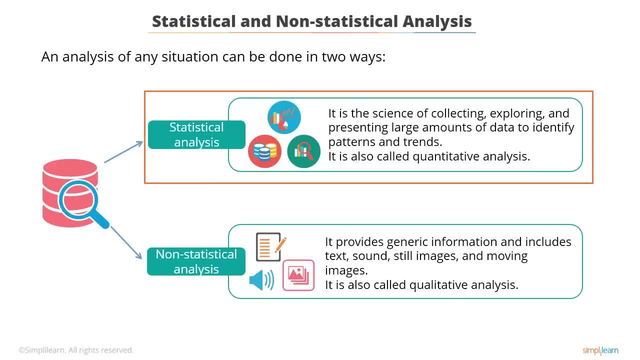 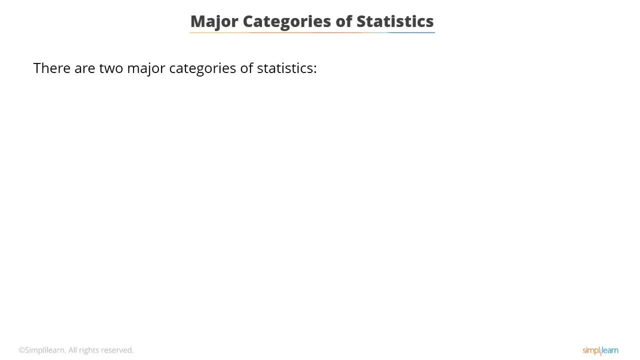 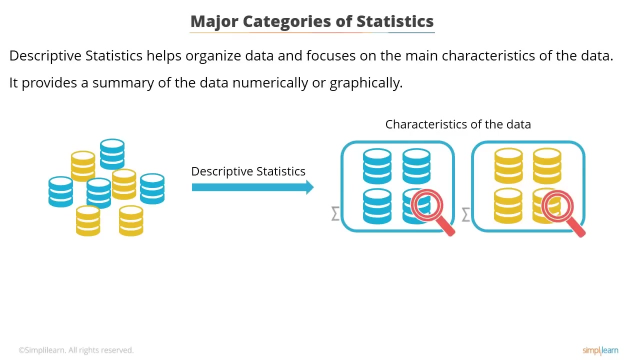 forms of analysis provide results. statistical analysis gives more insight and a clearer picture, a feature that makes it vital for businesses. There are two major categories of statistics: descriptive statistics and quantitative analysis. Statistical analysis provides a summary of the data numerically or graphically. Numerical measures, such as 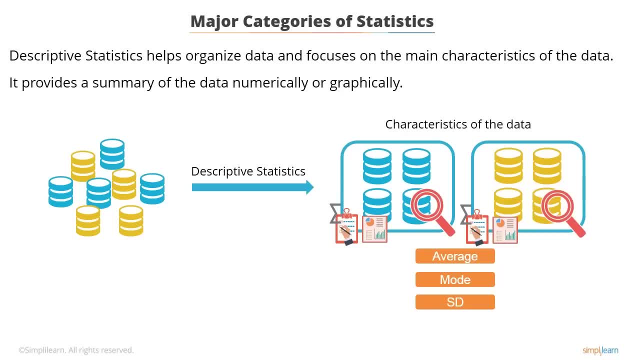 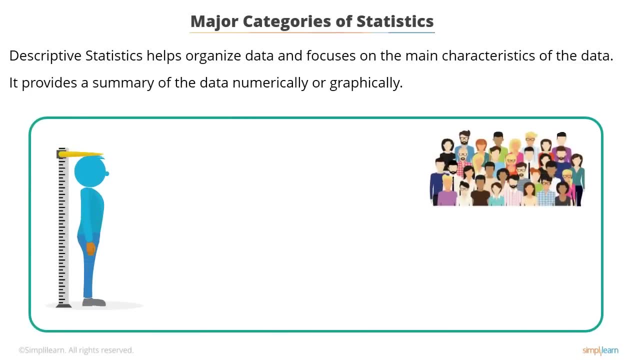 average mode, standard deviation or SD, and correlation are used to describe the features of a data set. Suppose you want to study the height of students in a classroom. In the descriptive statistics you would record the height of every person in the classroom. 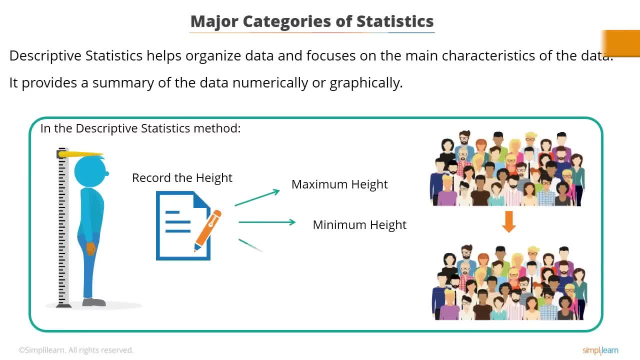 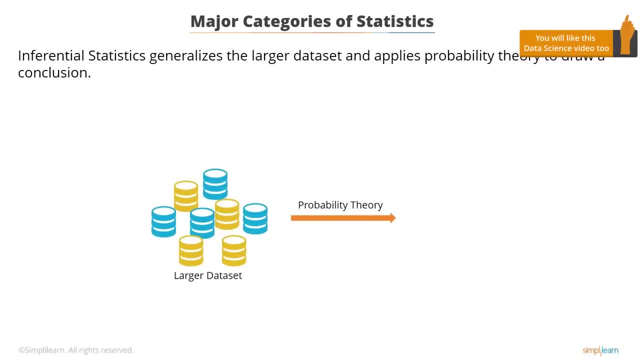 and then find out the maximum height, minimum height and average height of the population. Inferential statistics generalizes the larger data set and applies Probability theory. to draw a conclusion, It allows you to infer population parameters based on the sample statistics and to model relationships within the data. Modeling allows you to develop mathematical 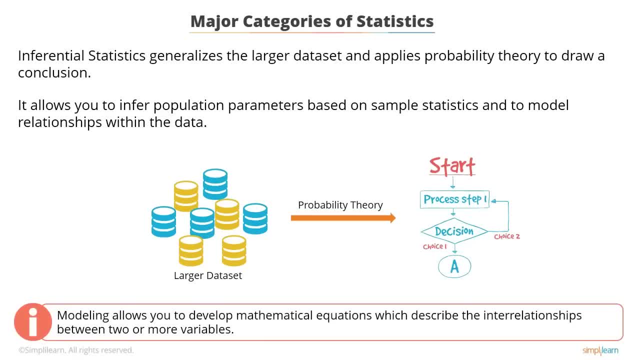 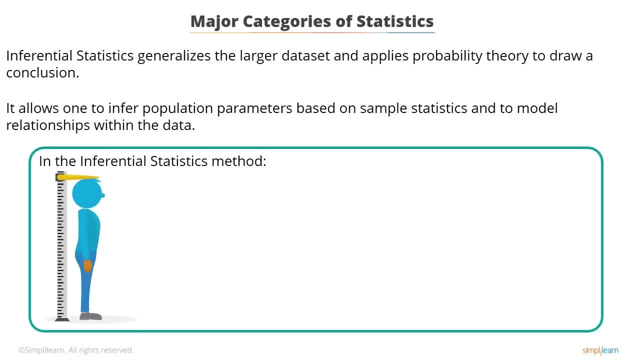 equations which describe the interrelationships between two or more variables. Consider the same example of calculating the distance between one and the other half of the clock using the height of students in the classroom. in inferential statistics you would categorize height as tall, medium and small, and then take only a small sample from the population. 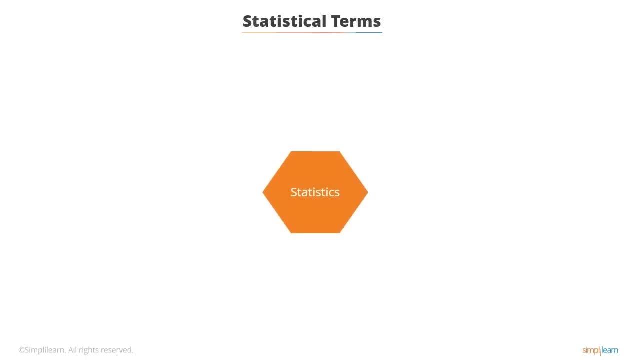 to study the height of students in the classroom. The field of statistics touches our lives in many ways. from the daily routines in our homes to the business of making the greatest cities run, the effect of statistics are everywhere. There are various statistical terms that one should be aware of while dealing with statistics. 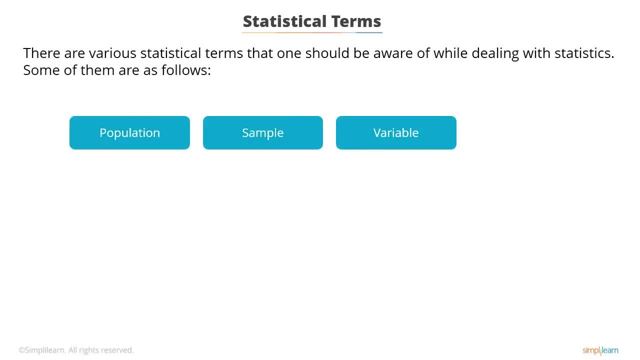 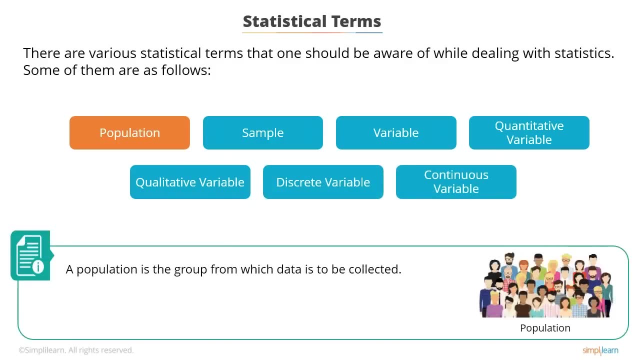 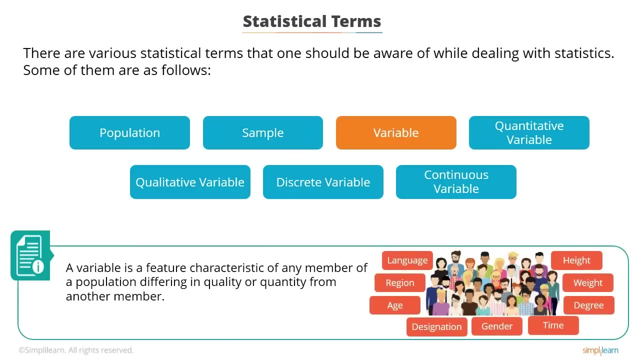 – population sample variable, quantitative variable, qualitative variable, discrete variable, continuous variable. A population is the group from which data is to be collected. A sample is a subset of a population. A variable is a feature that is characteristic of any member of the population: differing. 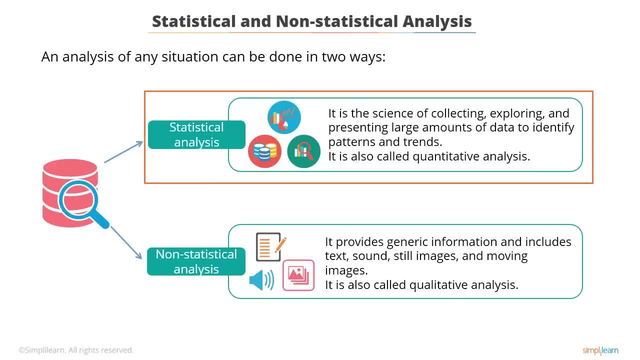 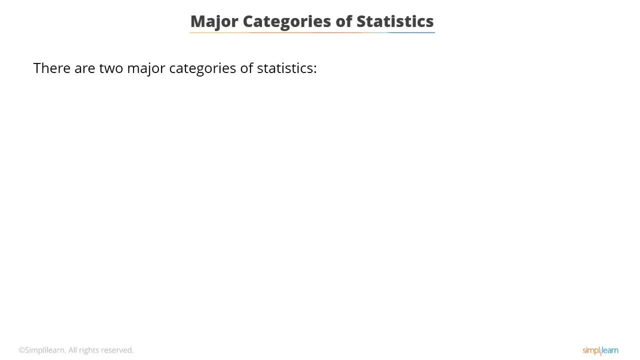 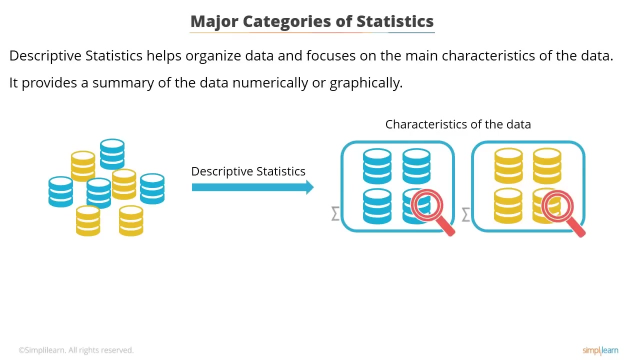 forms of analysis provide results. statistical analysis gives more insight and a clearer picture, a feature that makes it vital for businesses. There are two major categories of statistics: descriptive statistics and quantitative analysis. Statistical analysis provides a summary of the data numerically or graphically. Numerical measures, such as 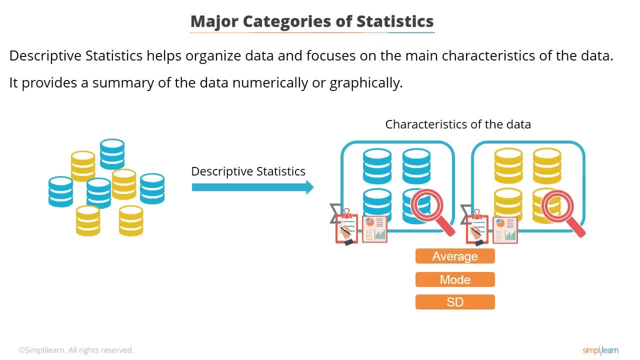 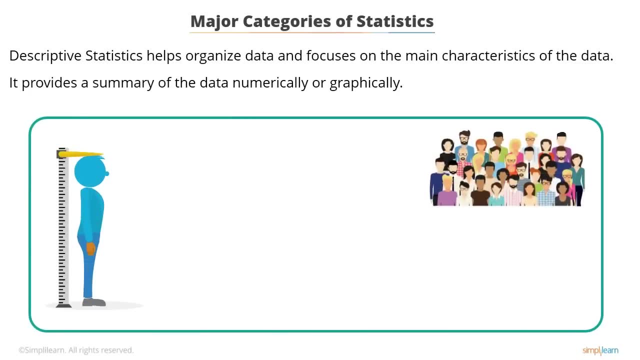 average mode, standard deviation or SD, and correlation are used to describe the features of a dataset. Suppose you want to study the height of students in a classroom. In the descriptive statistics you would record the height of every person in the classroom and then find out the maximum height, minimum height and average height. 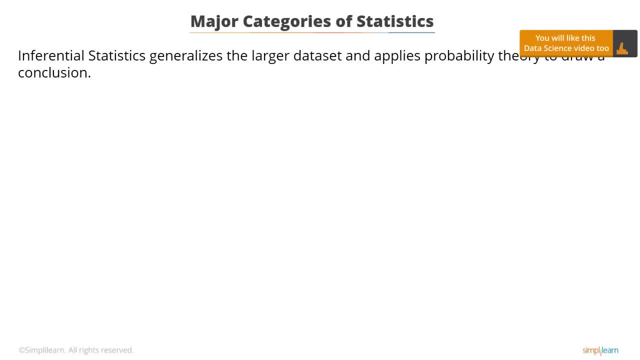 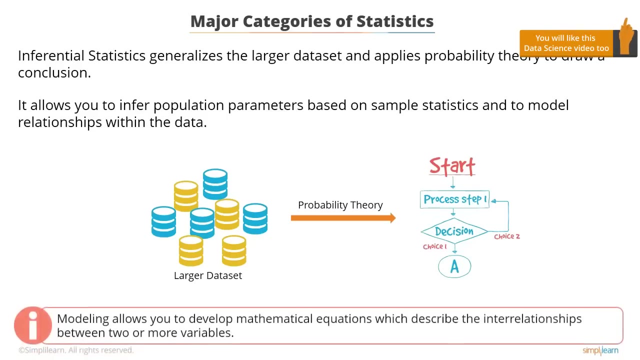 of the population. Inferential statistics generalizes the larger dataset and applies probability theory. to draw a conclusion, It allows you to infer population parameters based on the sample statistics and to model relationships within the data. Modeling allows you to develop mathematical equations which describe the interrelationships between two. 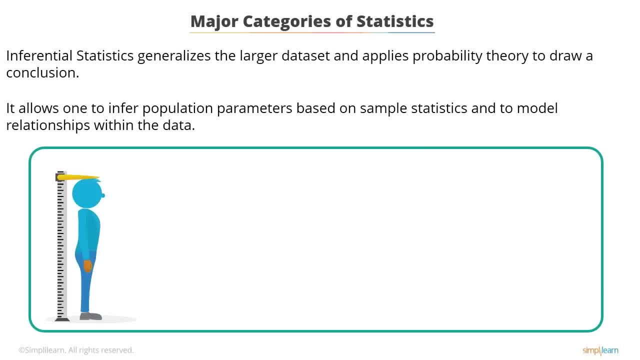 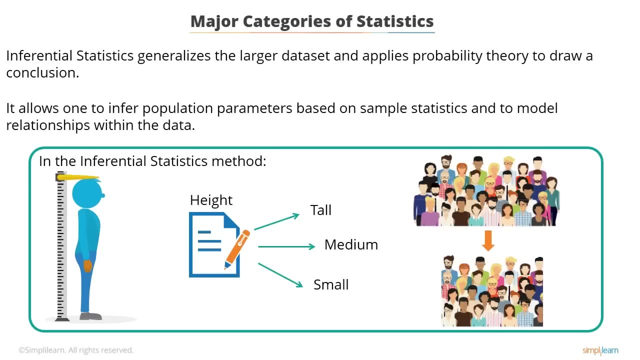 or more variables. Consider the same example of calculating the height of students in the classroom. In inferential statistics you would categorize height as tall, medium and small and then take only a small sample from the population to study the height of students in the classroom. 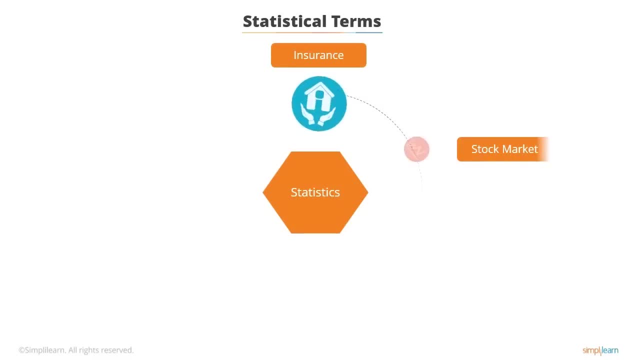 The field of statistics touches our lives in many ways. From the daily routines in our homes to the business of making the greatest cities run, the effect of statistics are everywhere. There are various statistical terms that one should be aware of while doing statistical work. The following are the number of variables that are used for population and population. 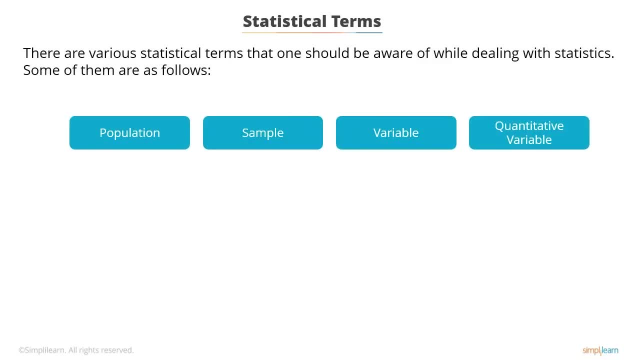 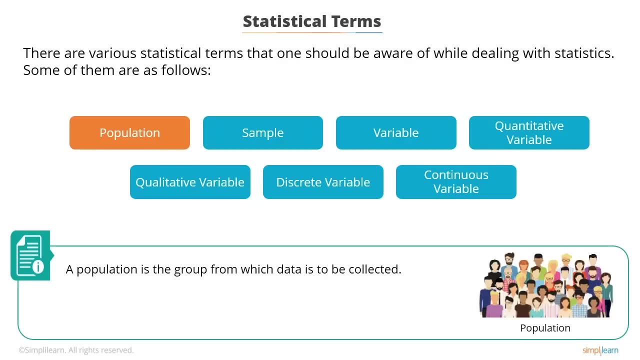 planning. There are 3 categories of population in the statistics: 1. Population, 2. Sample, 3. Variable, 4. Quantitative Variable. 5. Qualitative Variable. 6. Discrete Variable. 7. Continuous Variable. A population is the group from which data is to be collected. 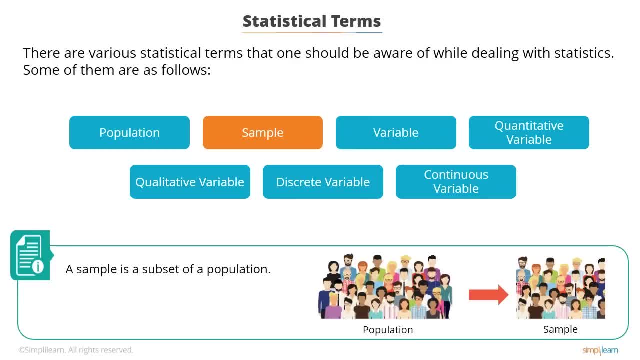 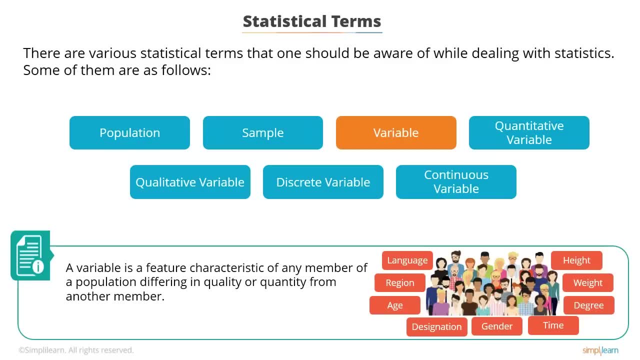 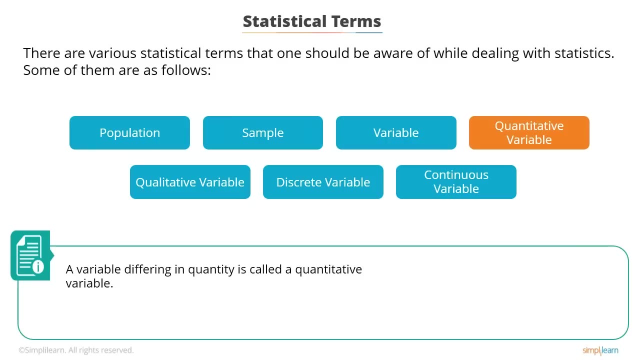 A sample is a subset of a population. A variable is a feature that is characteristic of any member of the population differing in quality or quantity from another member. A variable differing in quantity is called a quantitative variable. for example, the weight of a person, number of people in a car. 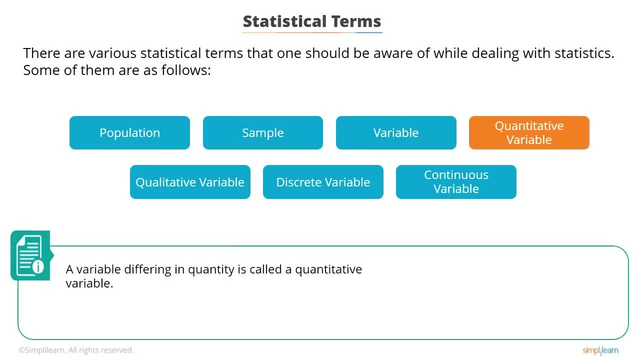 in quality or quantity from another member. A variable differing in quantity is called a quantitative variable, for example, the weight of a person, number of people in a car. A variable differing in quality is called a qualitative variable or attribute, for example, color, the degree of damage of a car in an accident. 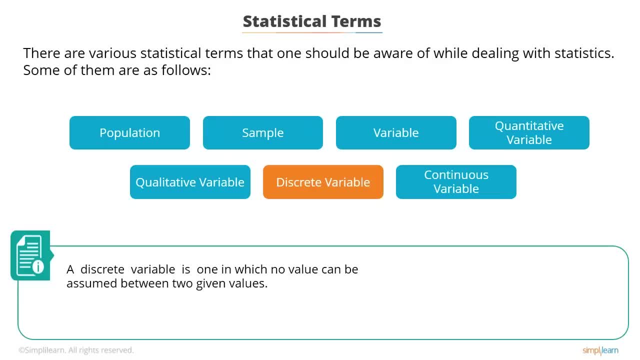 A discrete variable is one which no value can be assumed between the two given values, for example The number of children in a family. A continuous variable is one in which any value can be assumed between the two given values, for example the time taken for a 100-meter run. 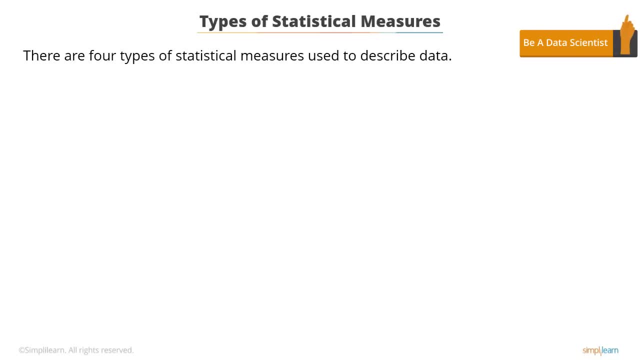 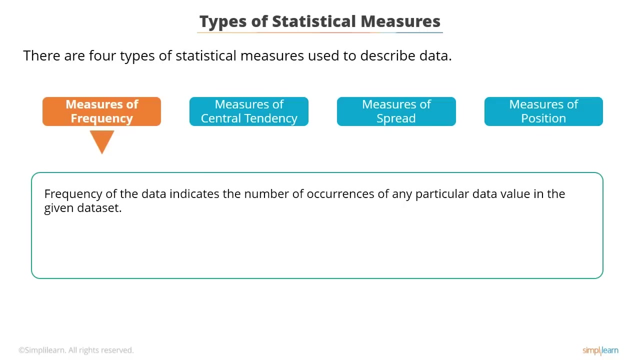 Typically, there are four types of statistical measures used to describe the data. They are measures of frequency, measures of central tendency, measures of spread, measures of position. Let's learn each in detail. Frequency of the data: It indicates the number of times a particular data value occurs in the given data set. 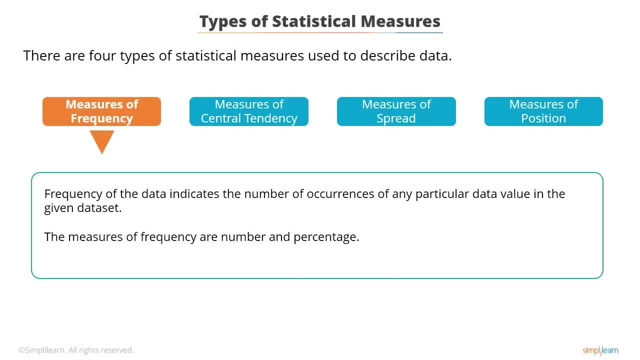 The measures of frequency are number and percentage. Central tendency indicates whether the data values tend to accumulate in the middle of the distribution or toward the end. The measures of central tendency are mean, median and mode. Spread describes how similar or varied the set of observed values are for a particular. 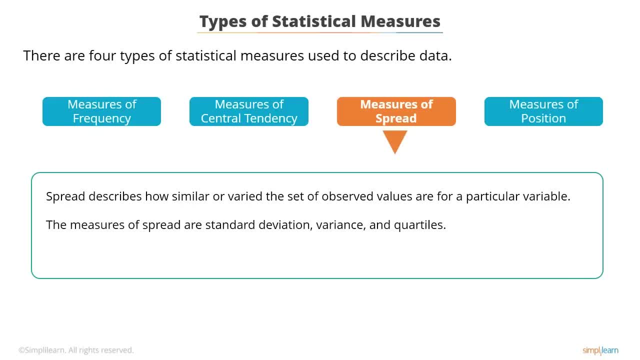 variable. The measures of spread are standard deviation Variants and quartiles. The measures of spread are also called measures of dispersion. Position identifies the exact location of a particular data value in the given data set. The measures of position are percentiles, quartiles and standard scores. 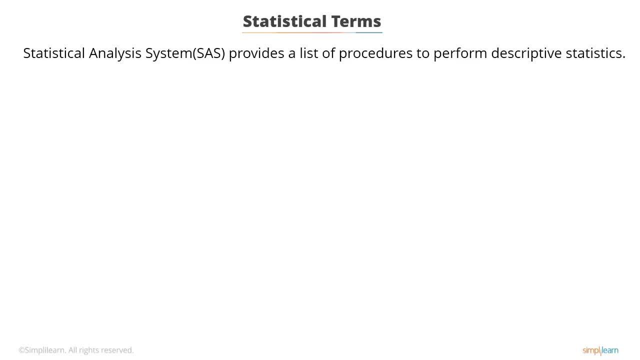 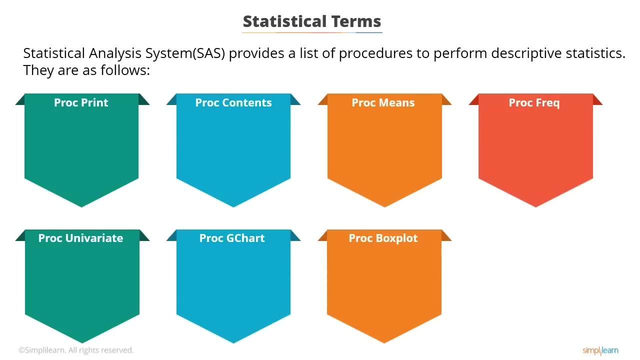 Statistical Analysis System, or SAS, provides a list of procedures to perform descriptive statistics. They are as follows: Proc print, Proc contents, Proc means, Proc frequency Proc univariate Proc. gchart, Proc boxplot, Proc gplot. Proc print. 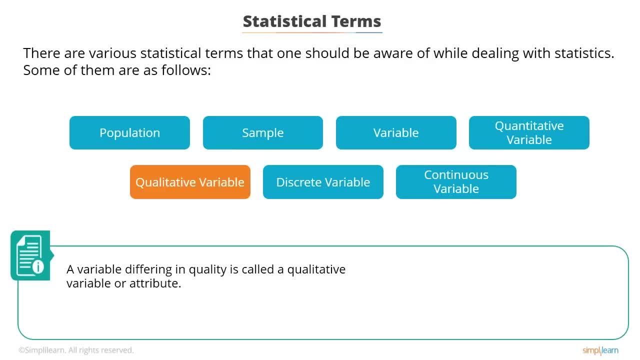 A variable differing in quality is called a qualitative variable or attribute, for example, color, the degree of damage of a car in an accident. A discrete variable is one which no value can be assumed between the two given values, for example the number of children in a family. 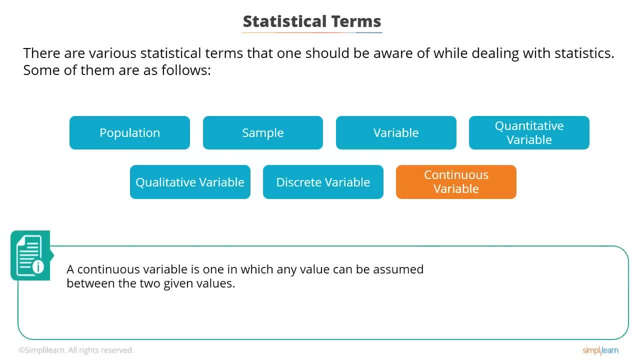 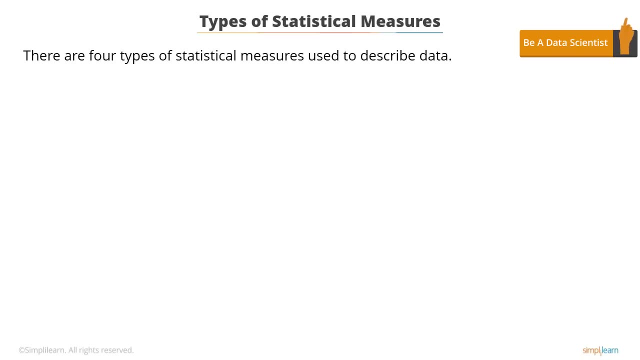 A continuous variable is one in which any value can be assumed between the two given values, for example, the time taken for a 100-meter run. Typically, there are four types of statistical measures used to describe the data. They are measures of frequency, measures of central tendency, measures of spread, measures of position. 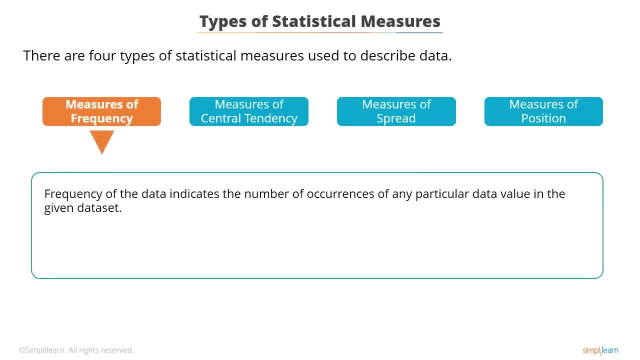 Let's learn each in detail. Frequency of the data indicates the number of times a particular event occurs, The number of times a particular data value occurs in the given data set. The measures of frequency are number and percentage. Central tendency indicates whether the data values tend to accumulate in the middle of the distribution or toward the end. 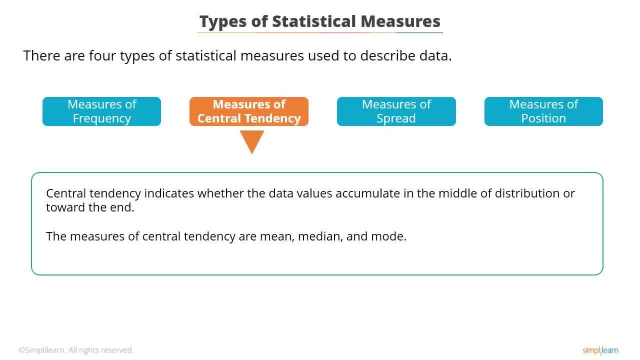 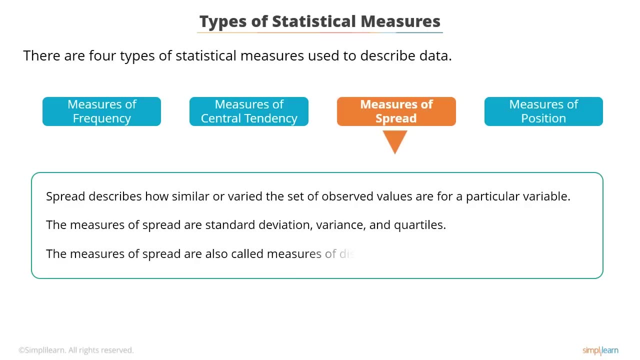 The measures of central tendency are mean, median and mode. Spread describes how similar or varied the set of observed values are for a particular variable. The measures of spread are standard, deviation, variance and quantity. The measures of spread are also called measures of dispersion. 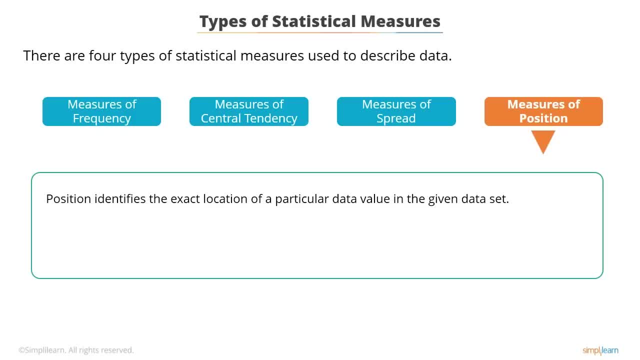 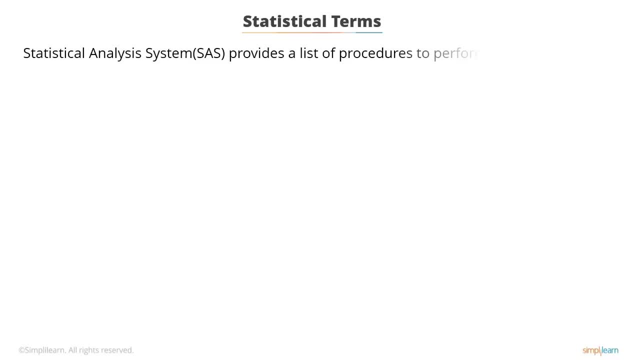 Position identifies the exact location of a particular data value in the given data set. The measures of position are percentiles, quartiles and standard scores. Statistical Analysis System, or SAS, provides a list of procedures to perform descriptive statistics. They are as follows. 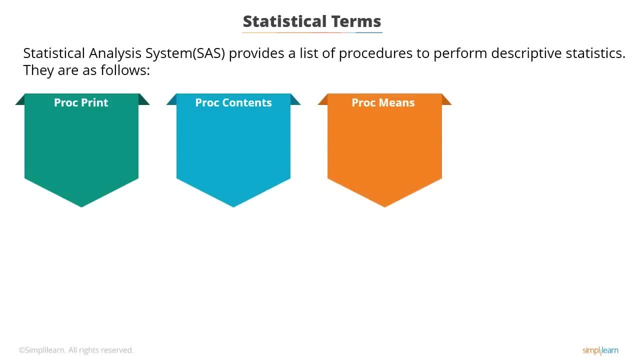 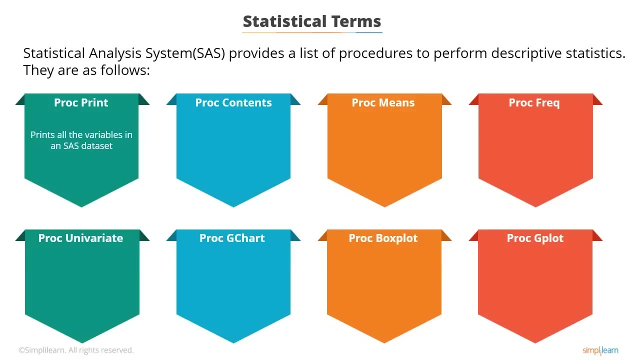 PROC PRINT- PROC CONTENTS. PROC MEANS. PROC FREQUENCY. PROC UNIVARIATE. PROC GCHART. PROC BOXPLOT. PROC GPLOT. PROC PRINT: It prints all the variables in a SAS data set. PROC CONTENTS: It describes the structure of a data set. 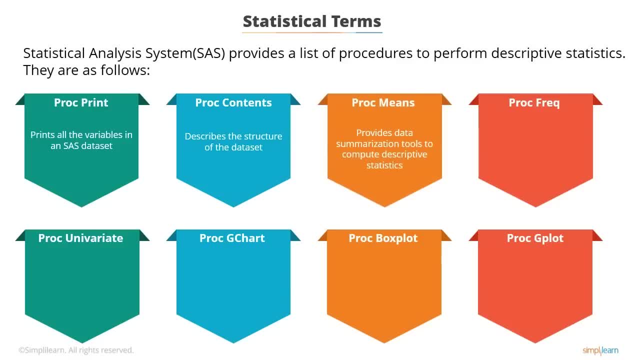 PROC MEANS: It provides data summarization tools to compute descriptive statistics for variables across all observations and within the groups of observations. PROC FREQUENCY: It produces one-way to n-way frequency and cross tabulation tables. Frequencies can also be an output of a SAS data set. 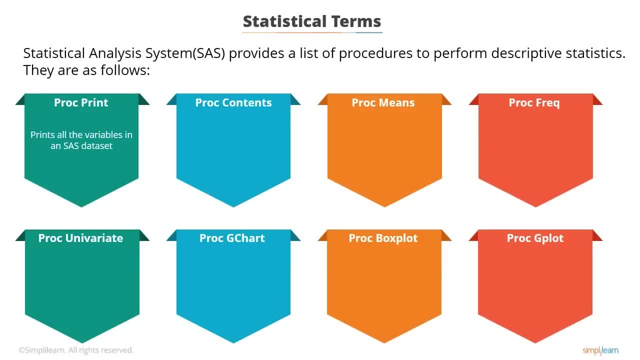 It prints all the variables in a SAS data set- Proc contents. It describes the structure of a data set- Proc means. It provides data summarization tools to compute descriptive statistics for variables across all observations and within the groups of observations- Proc means. 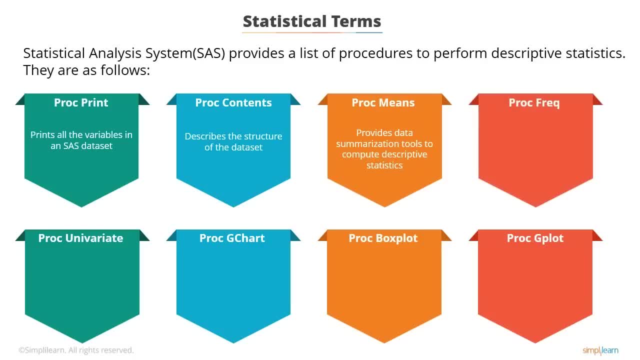 Proc means PROC FREQUENCY. It produces one-way to n-way frequency and cross-tabulation tables. Frequencies can also be an output of a SAS dataset, PROC UNIVARIATE. It goes beyond what PROC MEANS does and is useful in conducting some basic statistical analyses and includes high-resolution graphical features. 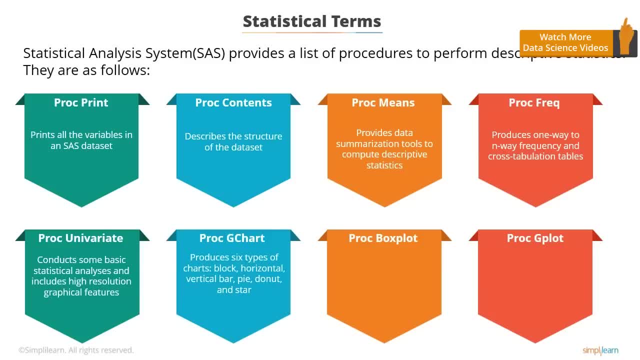 PROC GCHART. The gchart procedure produces six types of charts: block charts, horizontal vertical bar charts, pie donut charts and star charts. These charts graphically represent the value of a statistic calculated for one or more variables in an input SAS dataset. 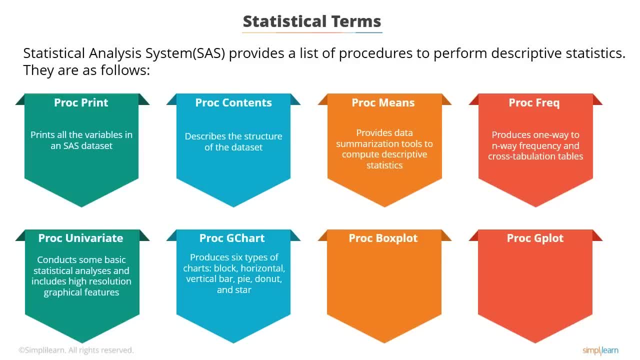 The charted variables can be either numeric or character. PROC BOXPLOT. The boxplot procedure creates side-by-side box-and-whisker plots of measurements organized. A box-and-whisker plot displays the mean quartiles and minimum and maximum observations for a group. 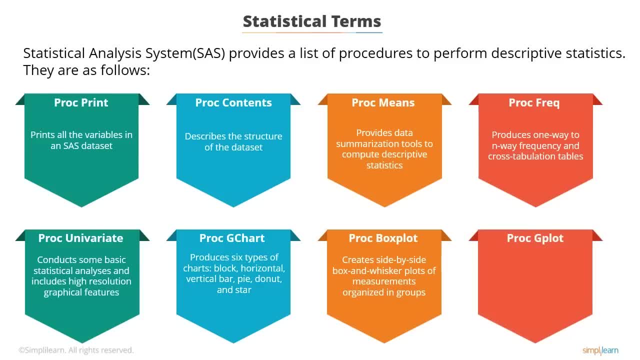 PROC GPLOT. The gplot procedure creates two-dimensional graphs including simple scatterplots, overlay plots in which multiple sets of data points are displayed on one set of axes, plots against a second vertical axis, bubble plots and logarithmic plots. In this demo, you'll learn how to use descriptive statistics. 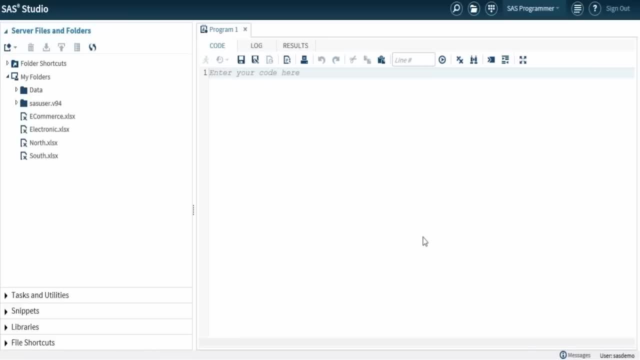 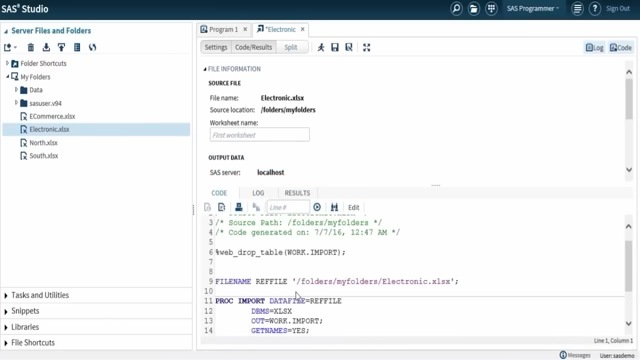 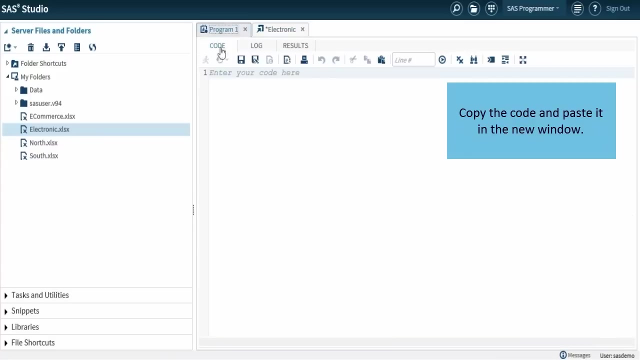 to analyze the mean from the electronic dataset. Let's import the electronic dataset into the SAS console. In the left plane, right-click the electronicxlsx dataset and click Import Data. The code to import the data generates automatically. Copy the code and paste it in the new window. 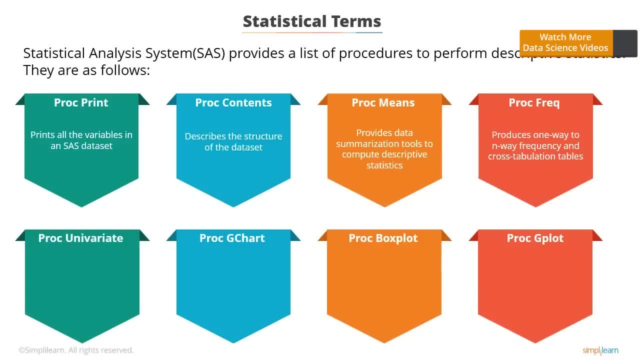 PROC UNIVARIATE. It goes beyond what PROC MEANS does and is useful in conducting some basic statistical analyses, and includes high-resolution graphical features. PROC GCHART: The GCHART procedure produces six types of charts: Block Charts, Horizontal Vertical Bar Charts, charts, pie-donut charts and star charts. 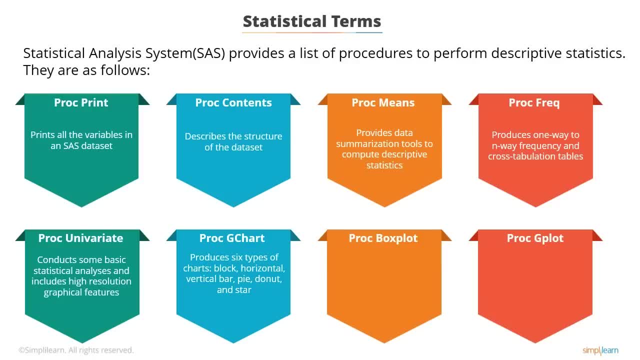 These charts graphically represent the value of a statistic calculated for one or more variables in an input SAS dataset. The charted variables can be either numeric or character. PROC BOXPLOT: The boxplot procedure creates side-by-side box-and-whisker plots of measurements organized in groups. 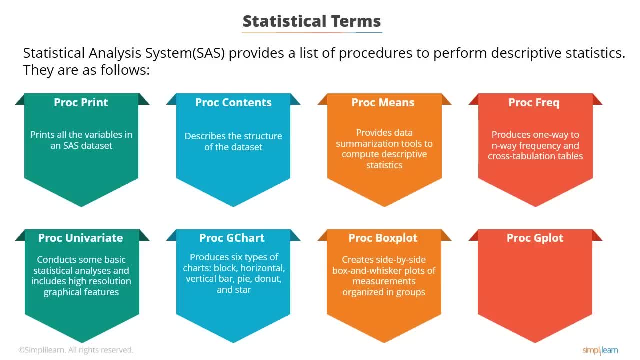 A box-and-whisker plot displays the mean, quartiles and minimum and maximum observations for a group. PROC GPLOT Gplot procedure creates two-dimensional graphs including simple scatter plots, overlay plots in which multiple sets of data points are displayed on one set of axes, plots against a second vertical axis, bubble plots and. 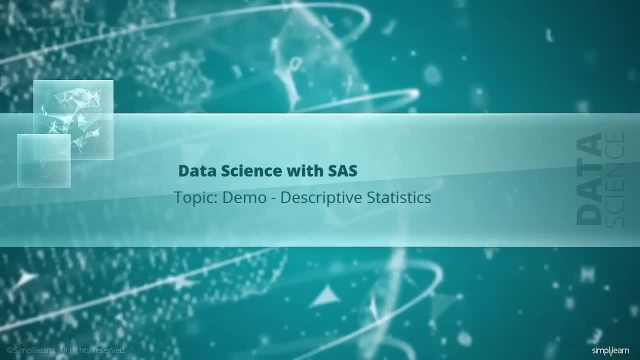 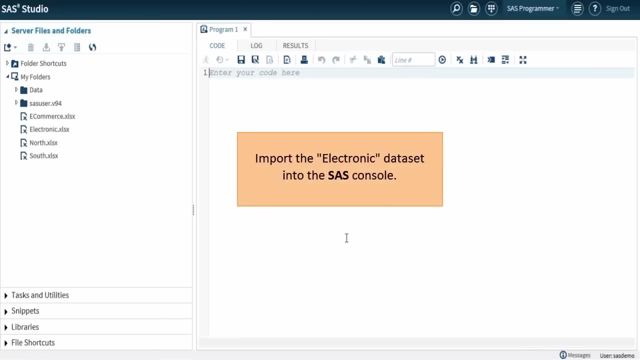 logarithmic plots. In this demo you'll learn how to use descriptive statistics to analyze the mean from the electronic dataset. Let's import the electronic dataset into the SAS console. In the left plane, right-click the electronicxlsx dataset and click Import Data. 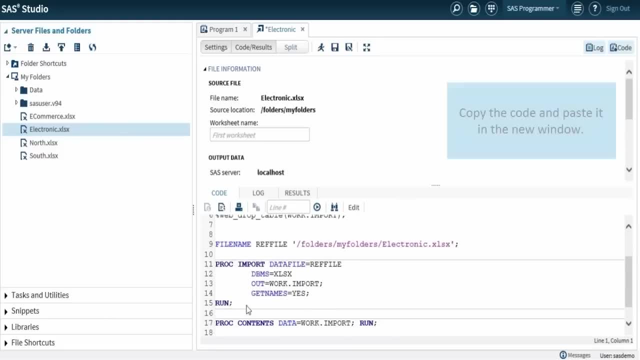 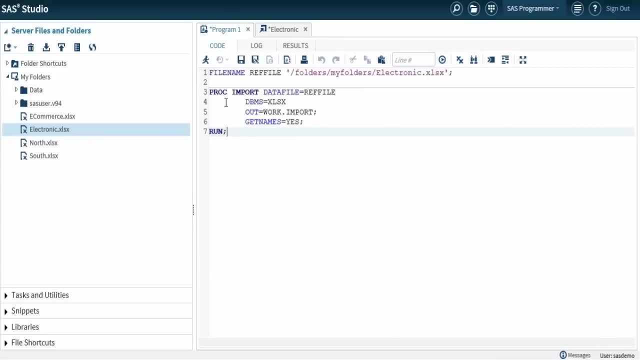 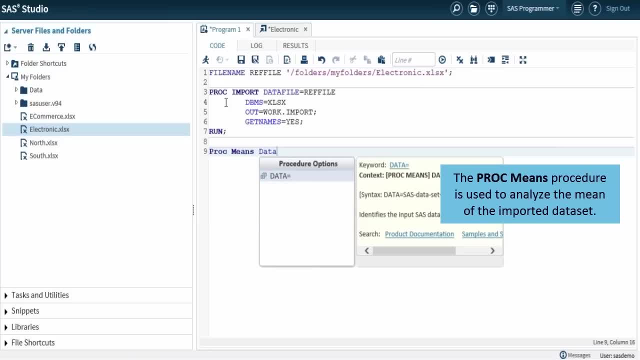 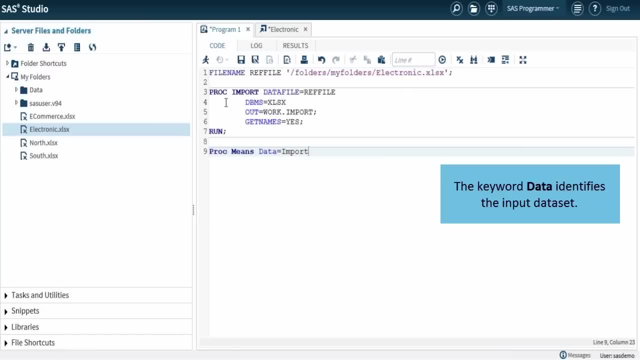 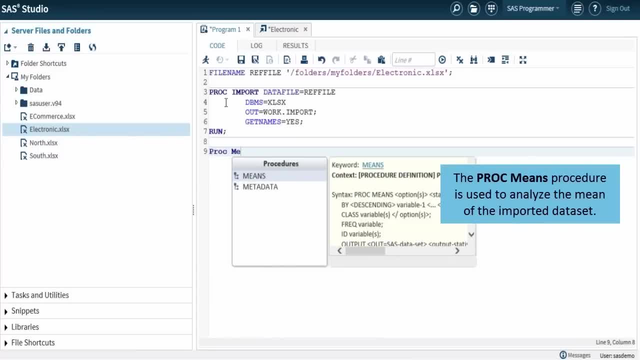 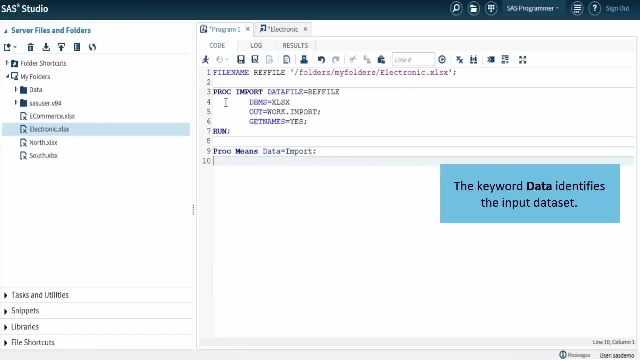 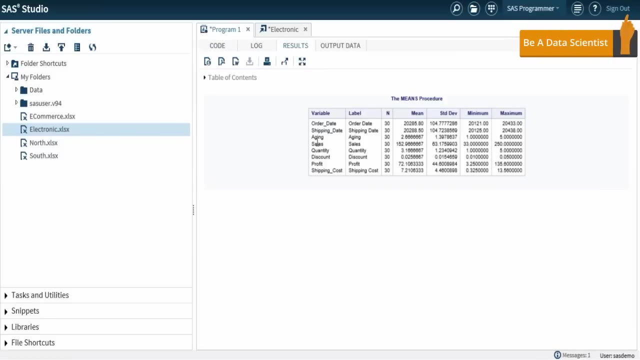 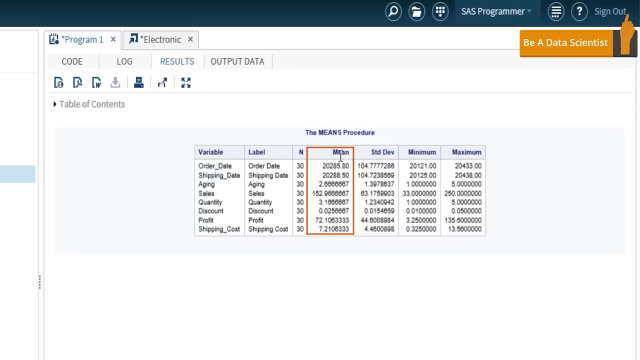 The PROC MEANS procedure is used to analyze the mean of the imported dataset. The keyword DATA identifies the input dataset. In this demo, the input dataset is electronic. The output obtained is shown on the screen. Note that the number of observations mean standard deviation. 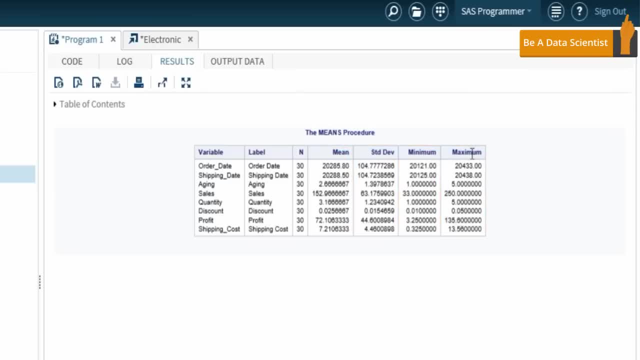 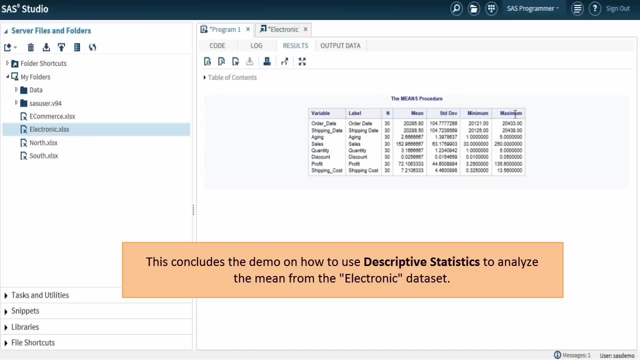 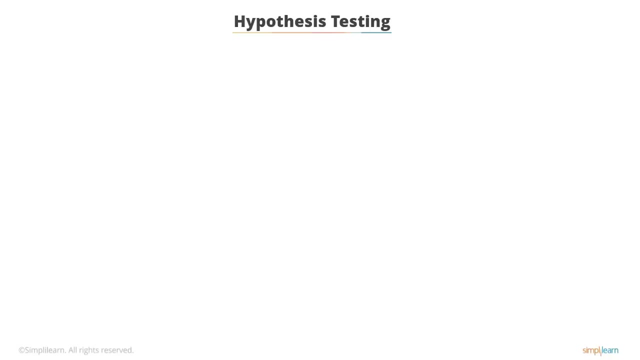 and maximum and minimum values of the electronic dataset are obtained. This concludes the demo on how to use descriptive statistics to analyze the mean from the electronic dataset. So far you have learned about descriptive statistics. Let's now learn about inferential statistics. Hypothesis testing is an inferential statistical technique. 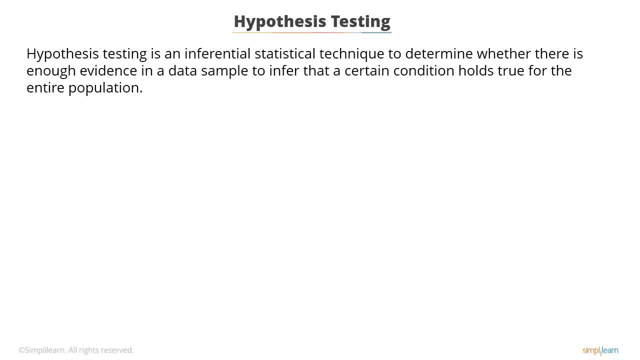 to determine whether there is enough evidence in a data sample to infer that a certain condition holds true for the entire population. To understand the characteristics of the general population, we take a random sample and analyze the properties of the sample. We then test whether or not the identified conclusions 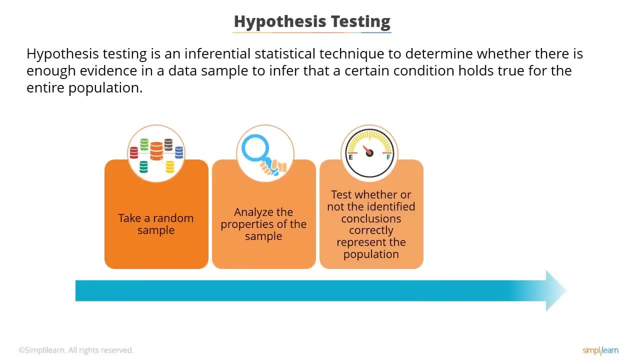 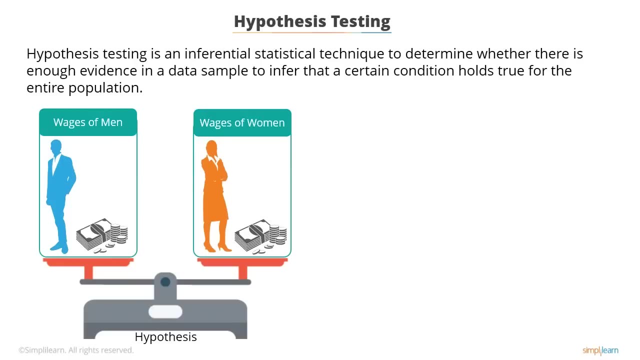 correctly represent the population as a whole. The population of hypothesis testing is to choose between two competing hypotheses about the value of a population parameter. For example, one hypothesis might claim that the wages of men and women are equal, while the other might claim that women make more than men. 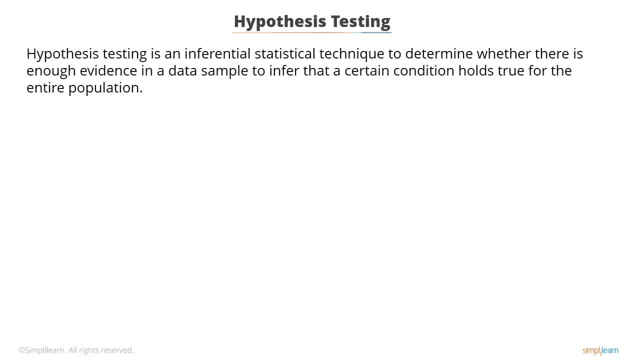 Hypothesis testing is formulated in terms of two hypotheses: Null hypothesis, which is referred to as H. null Alternative hypothesis, which is referred to as H1.. The null hypothesis is assumed to be true unless there is strong evidence to the contrary. 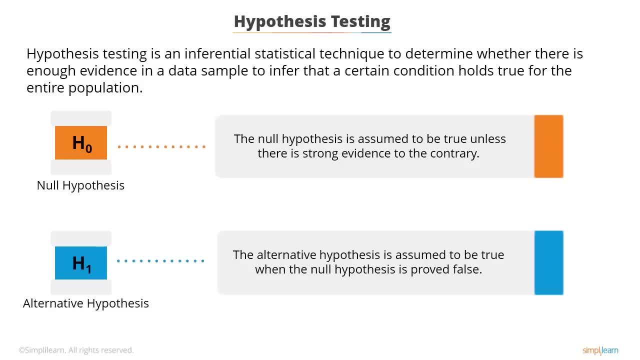 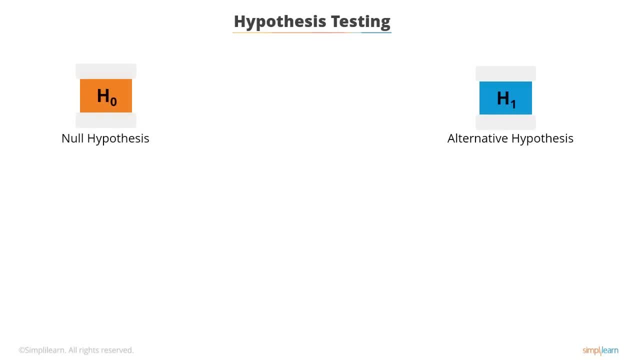 The alternative hypothesis is assumed to be true when the null hypothesis is proven false. Let's understand the null hypothesis and alternative hypothesis using a general example. Null hypothesis attempts to show that no variation exists between variables and alternative hypothesis. is any hypothesis other than the null? 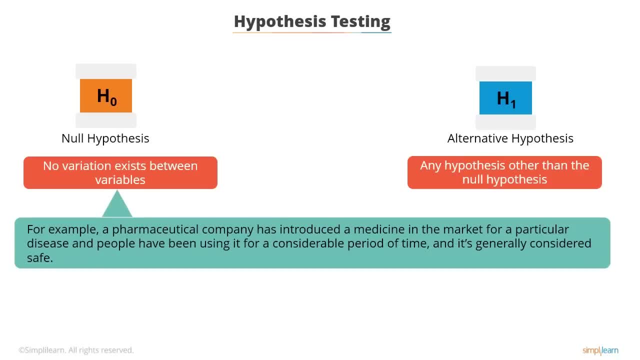 For example, say, a pharmaceutical company has introduced a medicine in the market for a particular disease and people have been using it for a considerable period of time and it's generally considered safe. If the medicine is proved to be safe, then it is referred to as null hypothesis. 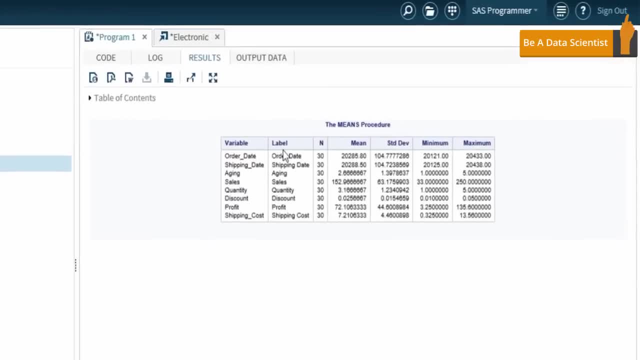 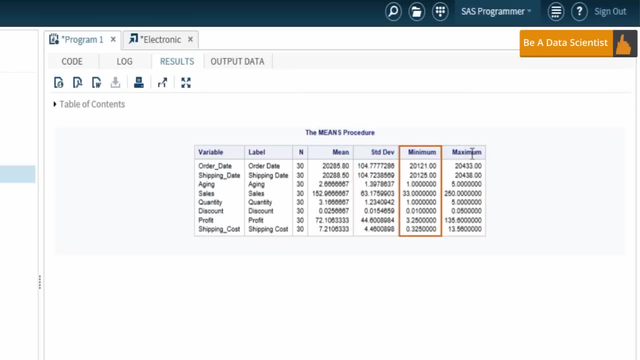 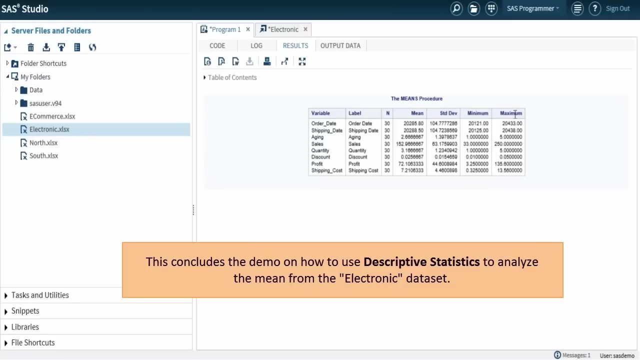 The output obtained is shown on the screen. Note that the number of observations, mean, standard deviation and maximum and minimum values of the electronic data set are obtained. This concludes the demo on how to use descriptive statistics to analyze the mean from the electronic data set. 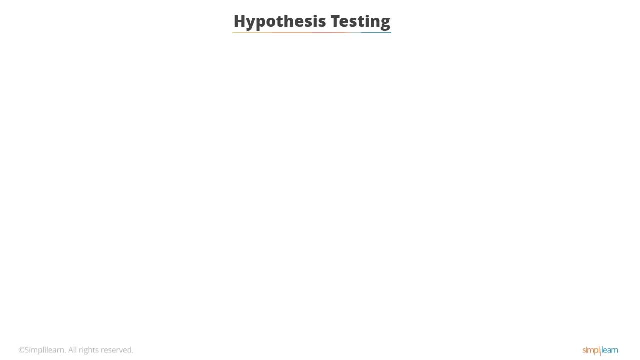 So far you have learned about descriptive statistics. Let's now learn about inferential statistics. Hypothesis testing is an inferential statistical technique to determine whether there is enough evidence in a data sample to infer that a certain condition holds true for the entire population. 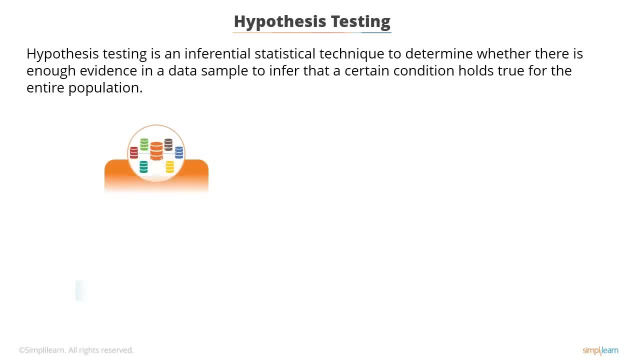 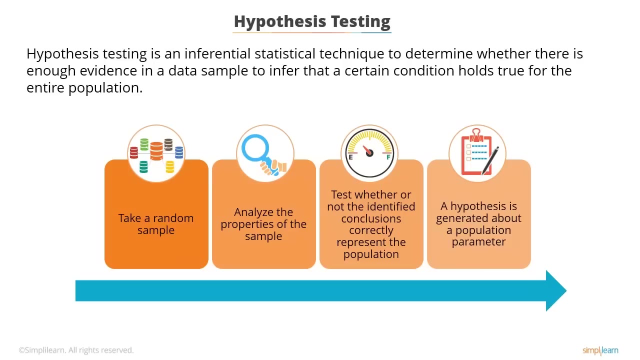 To understand the characteristics of the general population, we take a random sample and analyze the properties of the sample. We then test whether or not the identified conclusions correctly represent the population as a whole. The population of hypothesis testing is to choose between two competing hypotheses about the value. 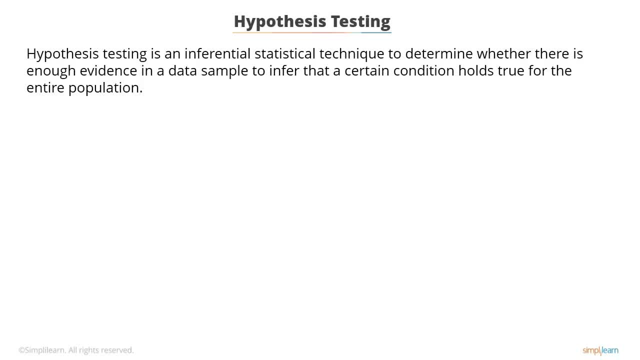 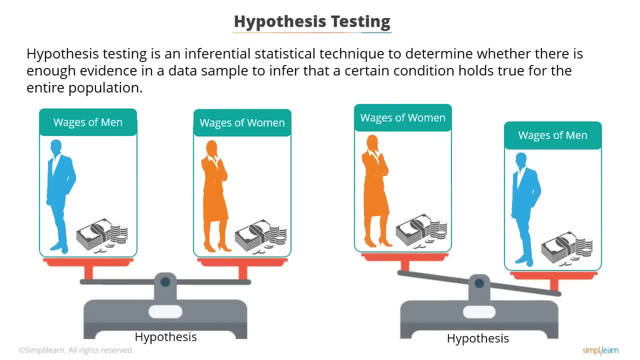 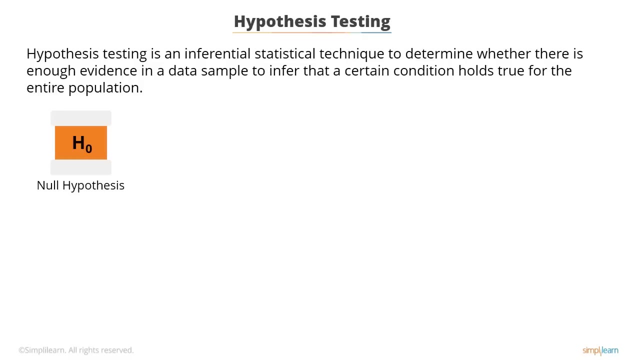 of a population parameter. For example, one hypothesis might claim that the wages of men and women are equal, while the other might claim that women make more than men. Hypothesis testing is formulated in terms of two hypotheses: Null hypothesis, which is referred to as H null. 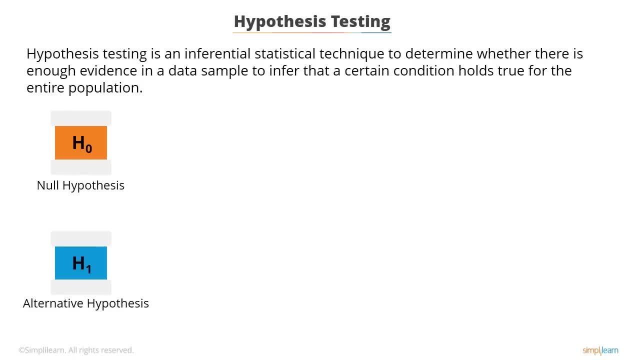 Alternative hypothesis, which is referred to as H1.. The null hypothesis is assumed to be true unless there is strong evidence to the contrary. The alternative hypothesis is assumed to be true when the null hypothesis is proven false. Let's understand the null hypothesis and alternative hypothesis using a general example. 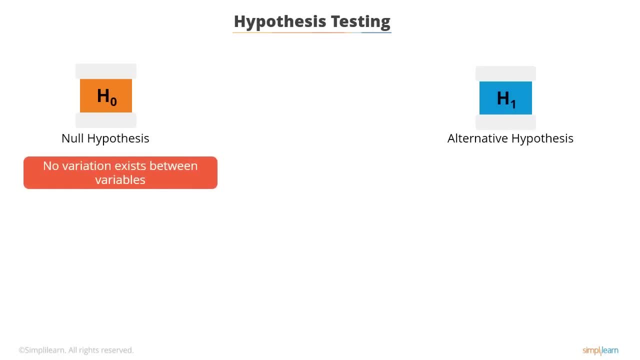 Null hypothesis attempts to show that no variation exists between variables and alternative hypothesis is any hypothesis other than the null. For example, Say, a pharmaceutical company has introduced a medicine in the market for a particular disease and people have been using it for a considerable period of time, and it's generally. 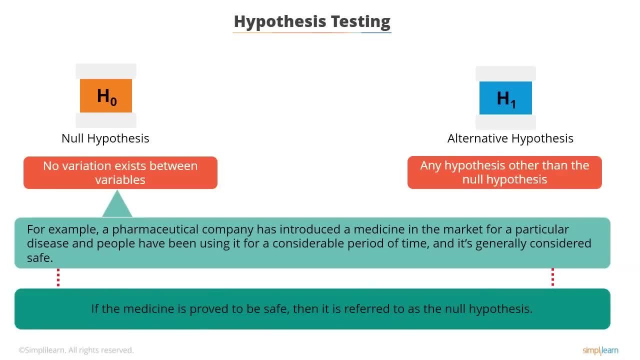 considered safe. If the medicine is proved to be safe, then it is referred to as null hypothesis. To reject null hypothesis, we should prove that the medicine is unsafe. If the null hypothesis is rejected, then the alternative hypothesis is used. 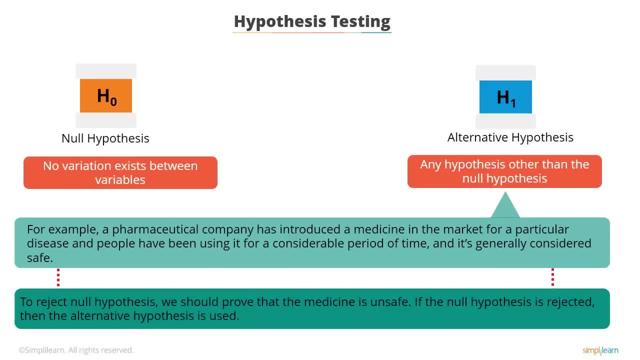 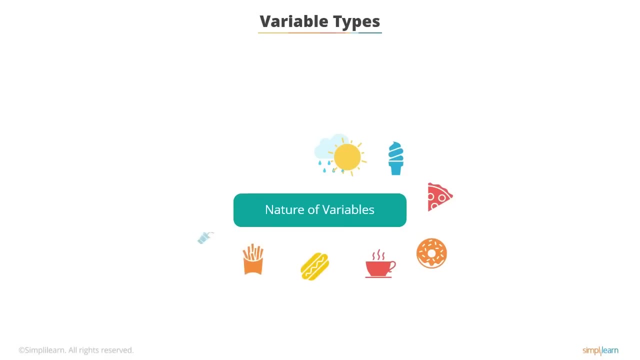 To reject null hypothesis, we should prove that the medicine is unsafe. If the null hypothesis is rejected, then the alternative hypothesis is used. Before you perform any statistical tests with variables, it's significant to recognize the nature of the variables involved. Based on the nature of the variables, 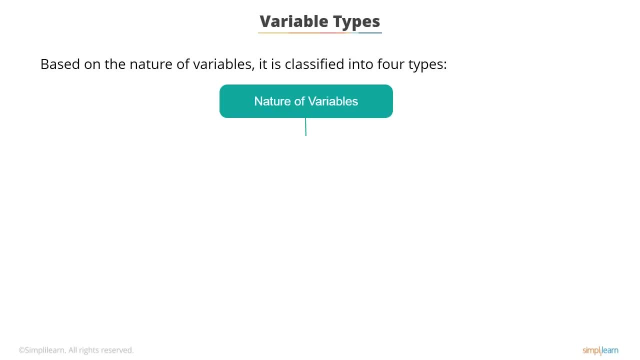 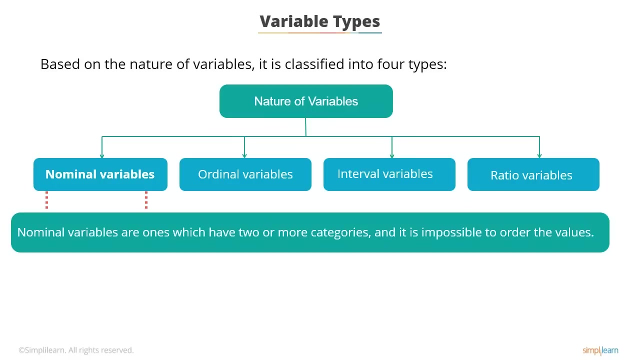 it's classified into four types. They are categorical or nominal variables, ordinal variables, interval variables and ratio variables. Nominal variables are ones which have two or more categories and it's impossible to order the values. Examples of nominal variables include gender and blood group. 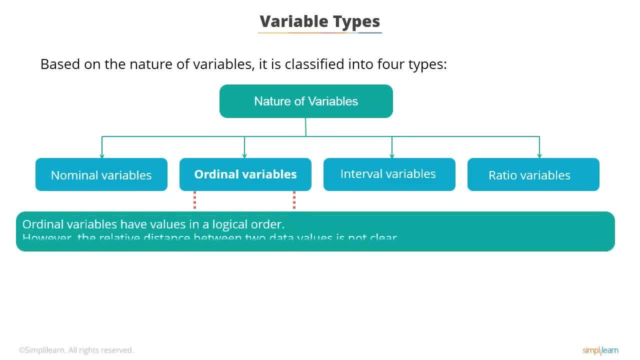 Ordinal variables have values ordered logically. However, the relative distance between two data values is not clear. Examples of ordinal variables include considering the size of a coffee cup- large, medium and small- and considering the ratings of a product- bad, good and best. 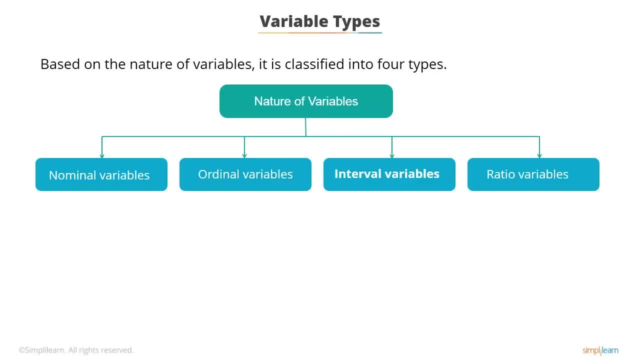 Interval variables are similar to ordinal variables, except that the values are measured in a way where their differences are meaningful. With an interval scale. equal differences between scale values do have equal quantitative meaning. For this reason, an interval scale provides more quantitative information than the ordinal scale. 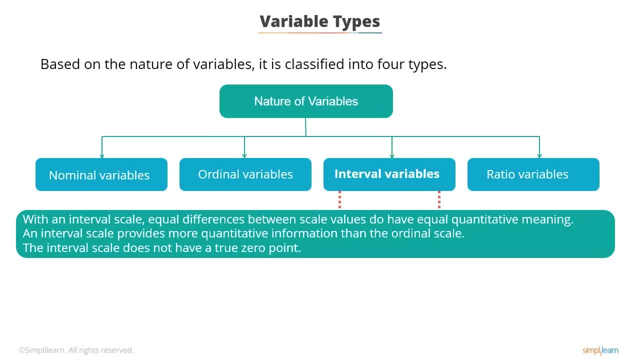 The interval scale does not have a true zero point. A true zero point means that a value of zero on the scale represents zero quantity of the construct being assessed. Examples of interval variables include the Fahrenheit scale used to measure temperature and distance between two compartments in a train. 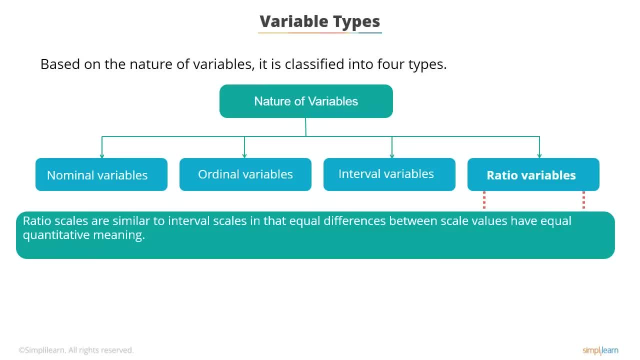 Ratio scales are similar to interval scales in that equal differences between scale values have equal quantitative meaning. However, ratio scales also have a true zero point, which give them an additional property. For example, the system of inches used with a common ruler is an example of a ratio scale. 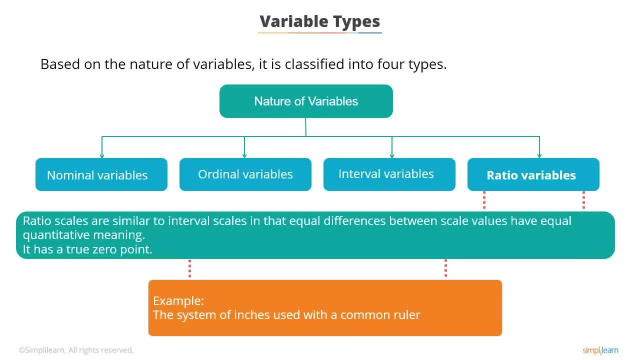 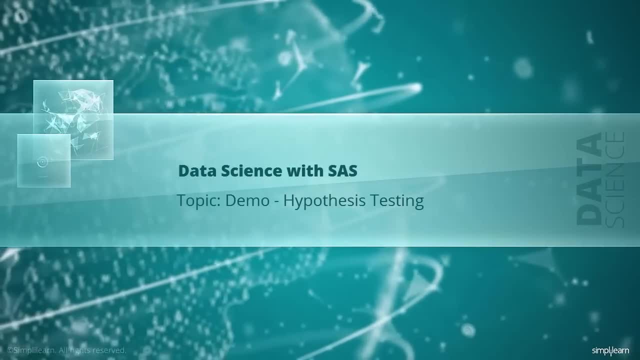 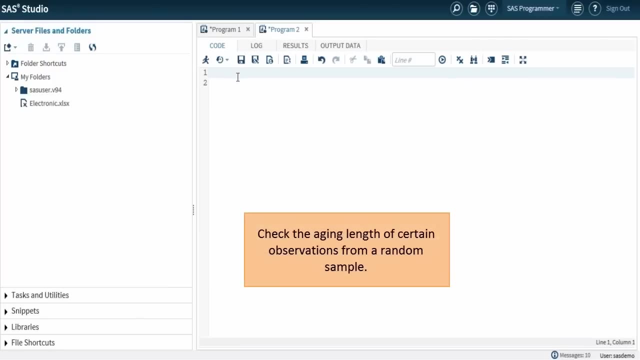 There is a true zero point, because zero inches does in fact indicate a complete absence of length. In this demo, you'll learn how to perform the hypothesis testing using SAS. In this example, let's check against the length of certain observations from a random sample. 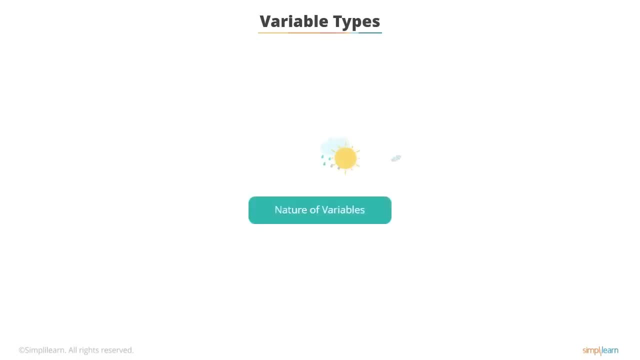 with variables, it's significant to recognize the nature of the variables involved. Based on the nature of the variables, it's classified into four types. They are categorical or nominal variables, ordinal variables, interval variables and ratio variables. Nominal variables are ones. 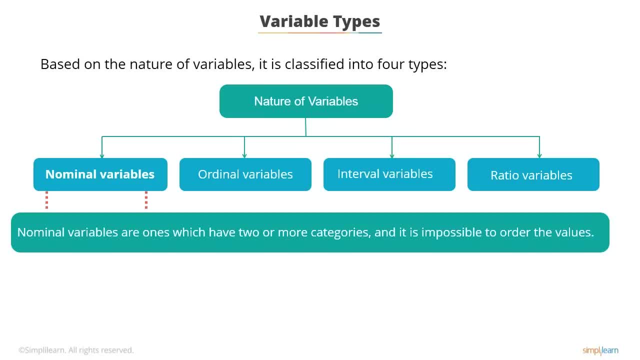 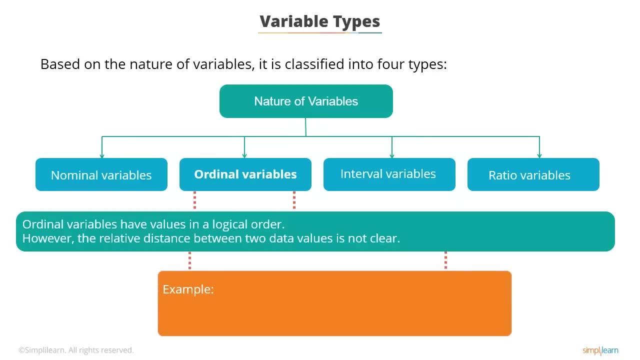 which have two or more categories and it's impossible to order the values. Examples of nominal variables include gender and blood group. Ordinal variables have values ordered logically. However, the relative distance between two data values is not clear. Examples of ordinal variables. 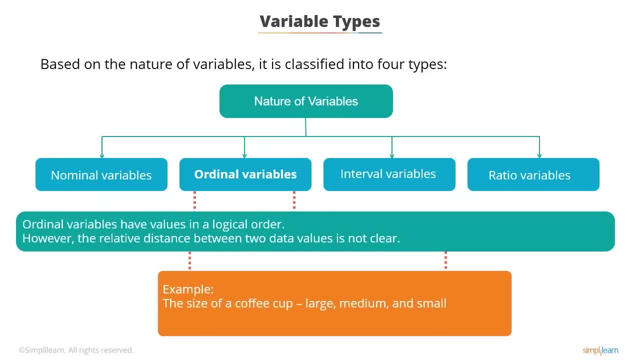 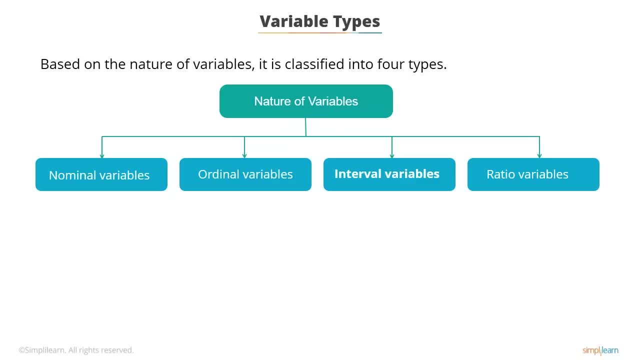 include considering the size of a coffee cup- large, medium and small- and considering the ratings of a product- bad, good and best. Interval variables are similar to ordinal variables, except that the values are measured in a way where their differences are meaningful. 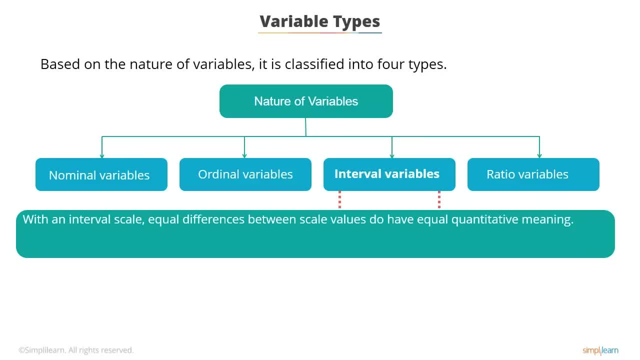 With an interval scale. equal differences between scale values do have equal quantitative meaning. For this reason, an interval scale provides more quantitative information than the ordinal scale. The interval scale does not have a true zero point. A true zero point means that a value of 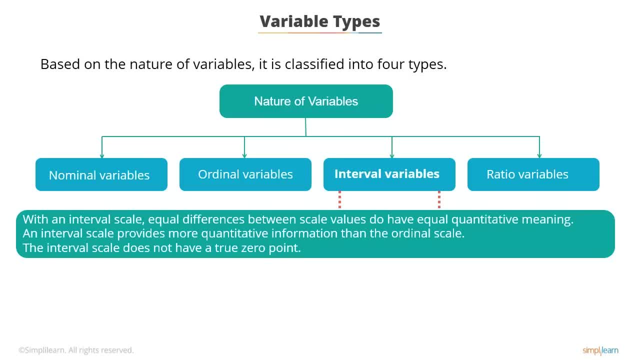 zero on the scale represents zero quantity of the construct being assessed. Examples of interval variables include: the Fahrenheit scale, used to measure temperature and distance between two compartments in a train. The interval scale is used to measure temperature and distance between two compartments in a train. 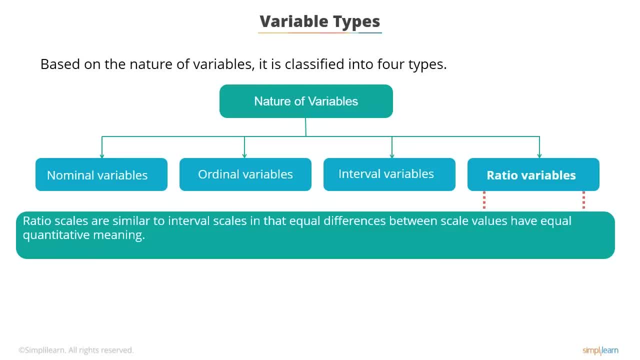 Ratio scales are similar to interval scales in that equal differences between scale values have equal quantitative meaning. However, ratio scales also have a true zero point, which gives them an additional property. For example, the system of inches used with a common ruler is an example of. 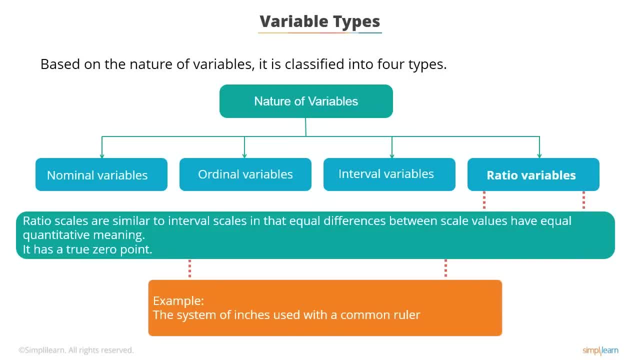 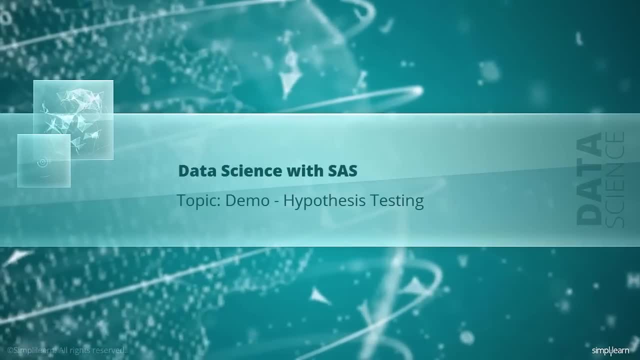 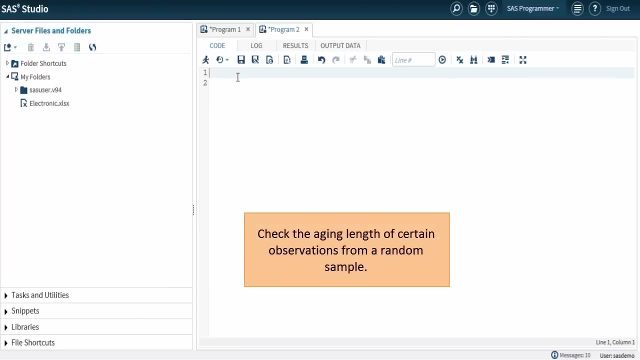 a ratio scale, There is a true zero point, because zero inches does in fact indicate a complete absence of length. In this demo, you'll learn how to perform the hypothesis testing using SAS. In this example, let's check against the length of certain observations from a random sample. 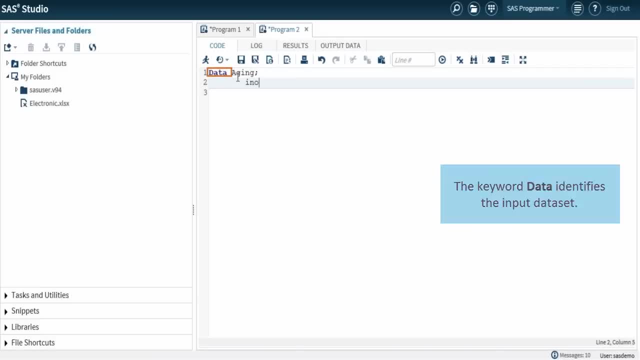 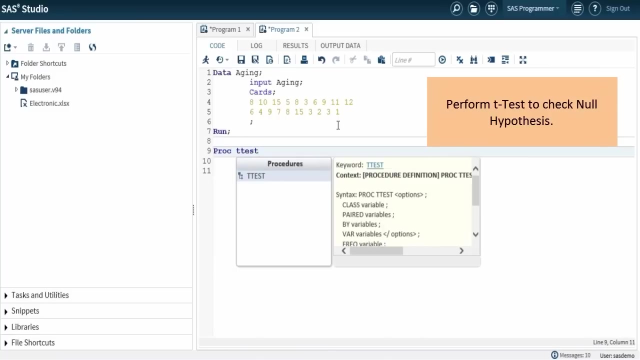 The keyword data identifies the input dataset. The input statement is used to declare the aging variable and cards to read data into SAS. Let's perform a t-test to check the null hypothesis. Let's assume that the null hypothesis to be that the mean days to deliver a product is six days. 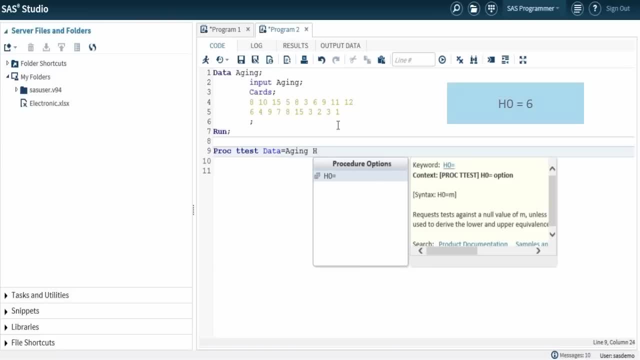 Let's assume that the null hypothesis to be that the mean days to deliver a product is six days. So null hypothesis equals six. Alpha value is the probability of making an error, which is five percent standard, and hence alpha equals zero point zero five. 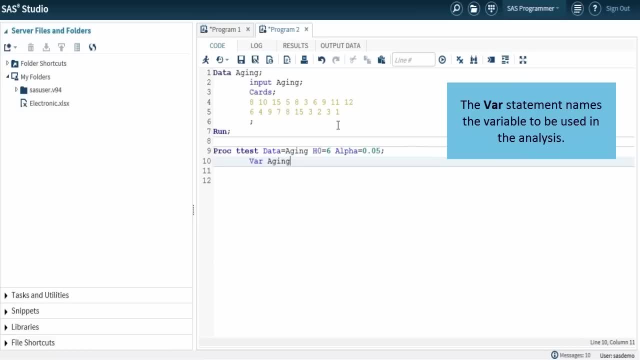 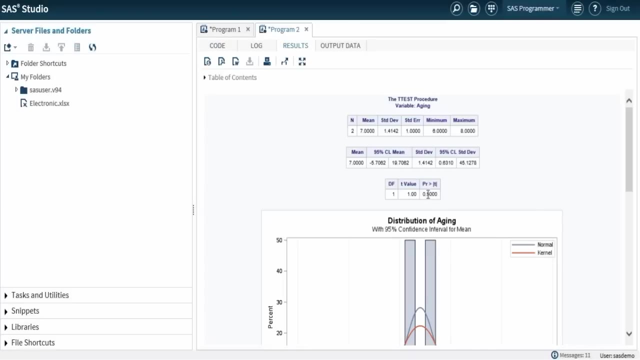 The variable statement names the variable to be used in the analysis. The output is shown on the screen. Note that the p-value is greater than the alpha value, which is zero point zero five. Therefore, we fail to reject the null hypothesis. This concludes the demo on how to perform the hypothesis testing using SAS. 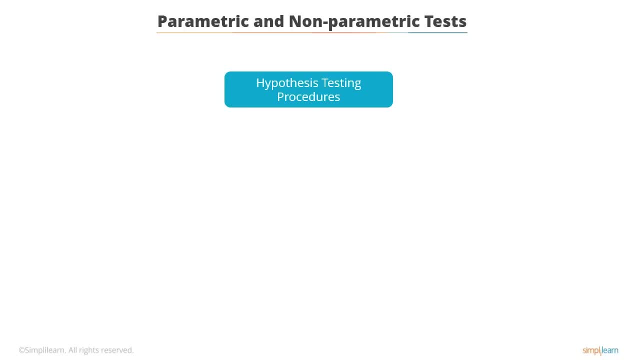 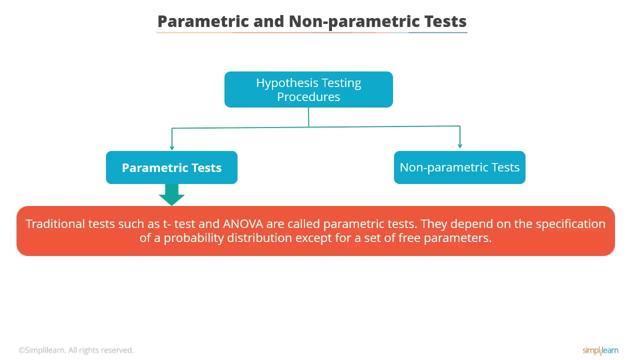 Let's now learn about hypothesis testing procedures. There are two types of hypothesis testing procedures. They are parametric tests and nonparametric tests. In statistical inference or hypothesis testing, the traditional tests, such as t-test and ANOVA, are called parametric tests. 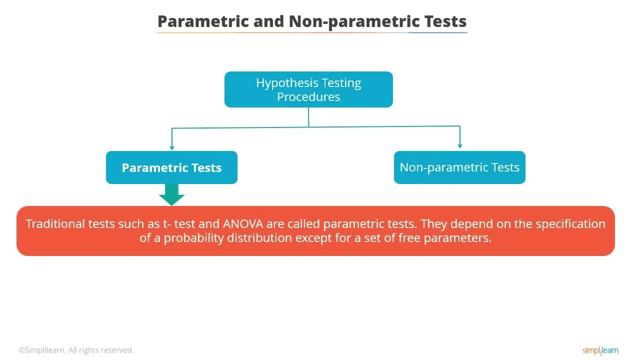 They depend on the specification of a probability distribution, except for a set of free parameters. In simple words, you can say that if the population information is known completely by its parameter, then it is called a parametric test. If the population or parameter information is not known, 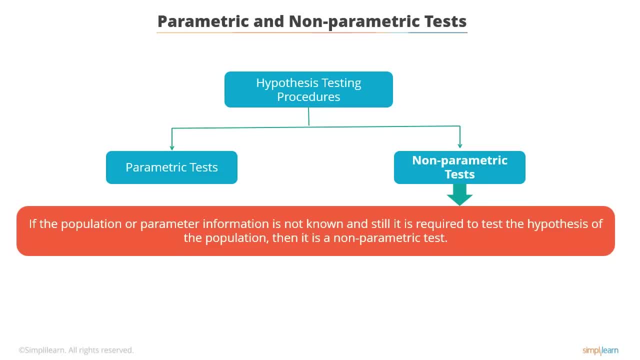 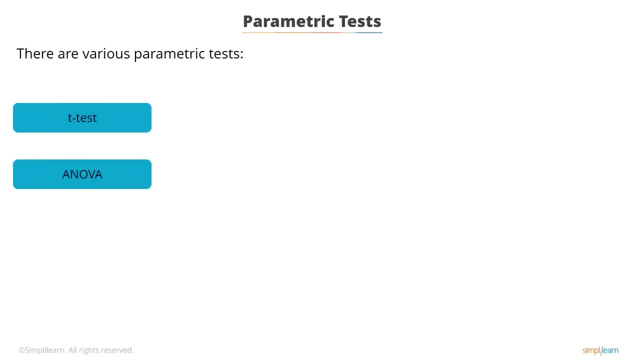 and you are still required to test the hypothesis of the population, then it is called a nonparametric test. Nonparametric tests do not require any strict distributional assumptions. There are various parametric tests. They are as follows: t-test, ANOVA, chi-squared linear regression. 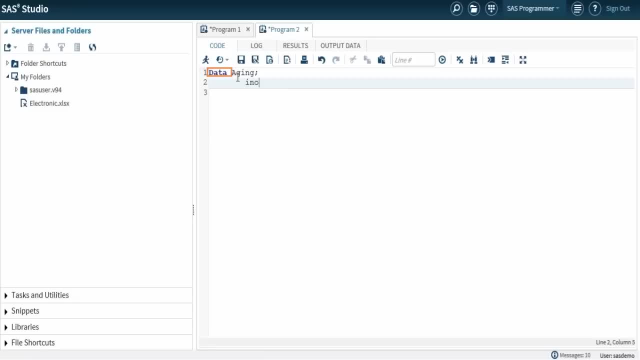 The keyword data identifies the input dataset. The input statement is used to declare the aging variable and cards to read data into SAS. We now search values in thedamnthedata technoetp to find out the output data. Let's perform a T-test to check the null hypothesis. 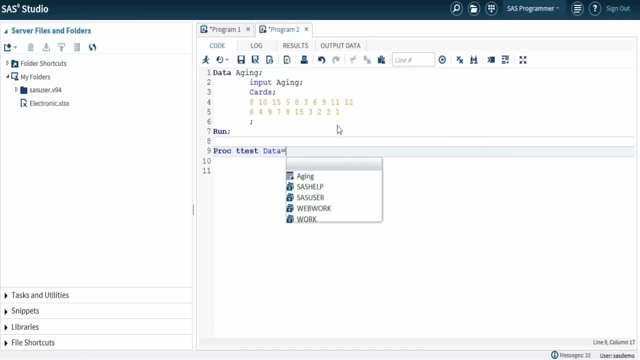 Let's assume that the null hypothesis is that the mean days to deliver a product is six days. So null hypothesis equals sixα value is the probability of making an error, which is 5% standard and hence alpha equals 0.05.. 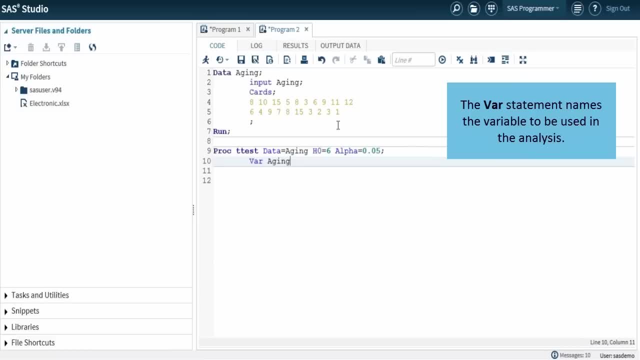 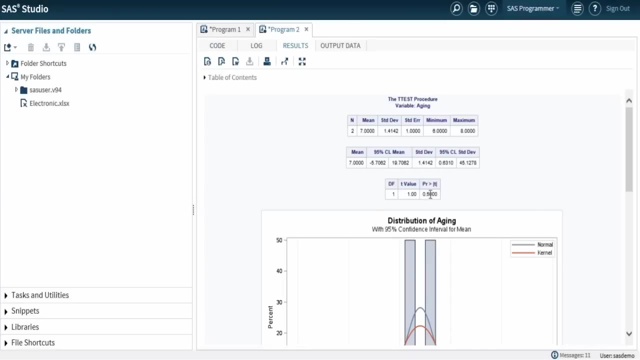 The variable statement names the variable to be used in the analysis. The output is shown on the screen. Note that the p-value is greater than the alpha value, which is 0.05.. Therefore, we fail to reject the null hypothesis. This concludes the demo on how to perform the hypothesis testing using SAS. 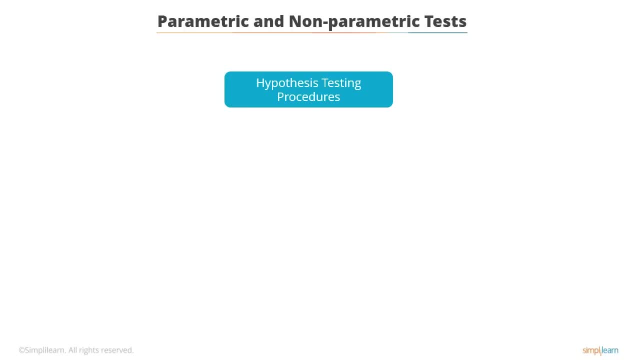 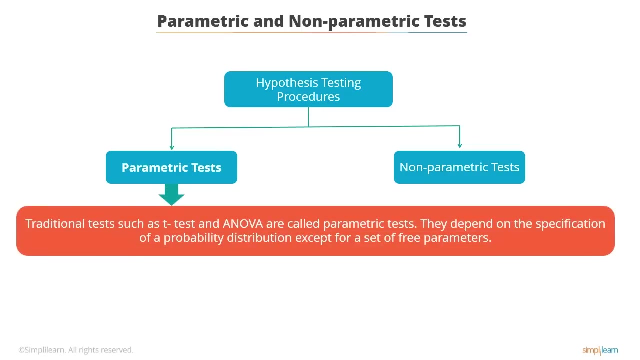 Let's now learn about hypothesis testing procedures. There are two types of hypothesis testing procedures. They are parametric tests and nonparametric tests. In statistical inference or hypothesis testing, the traditional tests, such as t-test and ANOVA, are called parametric tests. 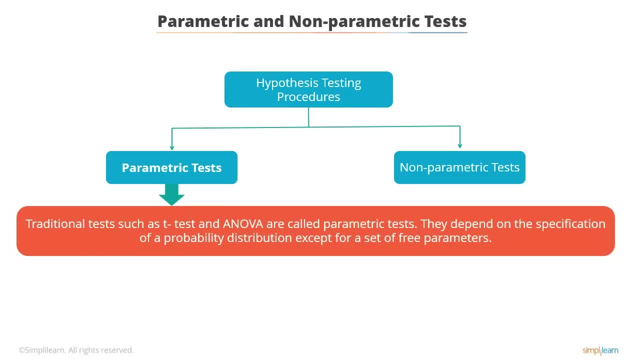 They depend on the specification of a probability distribution, except for a set of free parameters. In simple words, you can say that if the population information is known completely by its parameter, then it is called a parametric test. If the population or parameter information is not known, 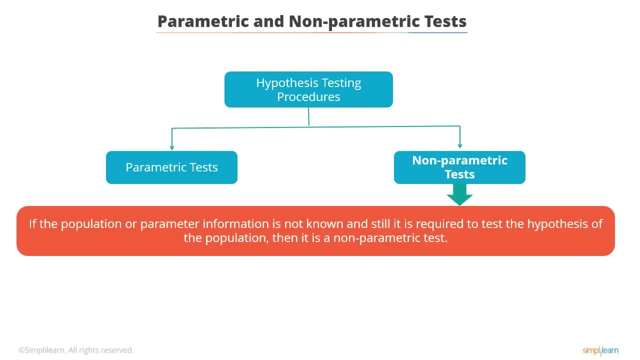 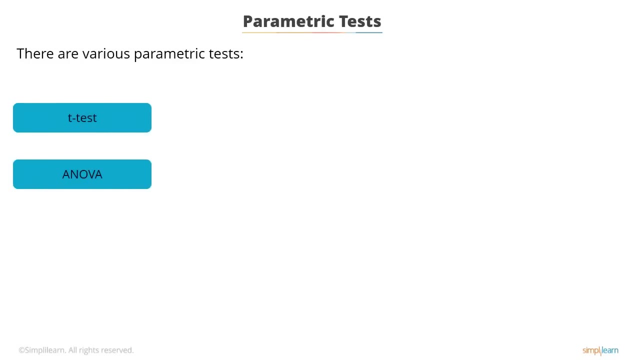 and you are still required to test the hypothesis of the population, then it is called a nonparametric test. Nonparametric tests do not require any strict distributional assumptions. There are various parametric tests. They are as follows: t-test, ANOVA, chi-squared linear regression. 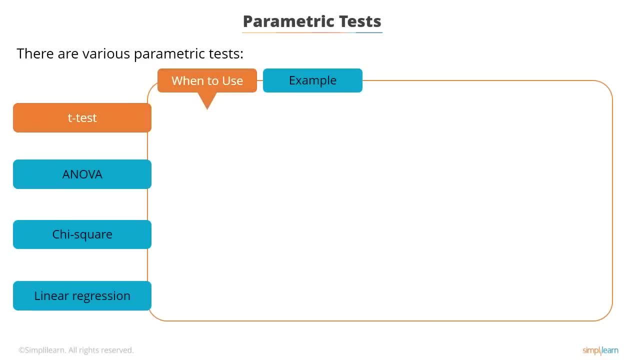 Let's understand them in detail. t-test: A t-test determines if two sets of data are significantly different from each other. The t-test is used in the following situations: To test if the mean is significantly different than a hypothesized value. To test if the mean for two independent groups is significantly different. 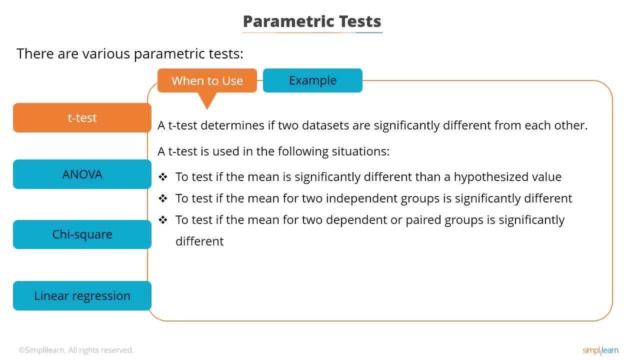 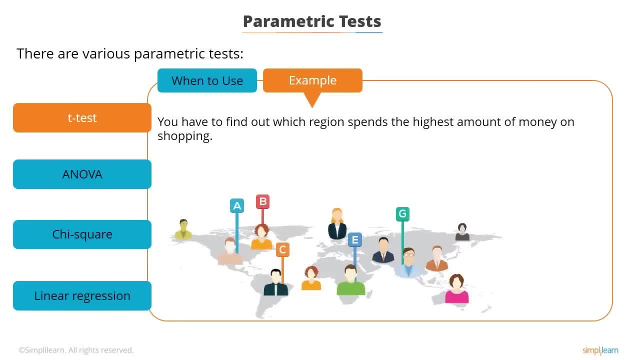 To test if the mean for two dependent or paired groups is significantly different. For example, let's say you have to find out which region spends the highest amount of money on shopping. It's impractical to ask everyone in the different regions about their shopping expenditure. 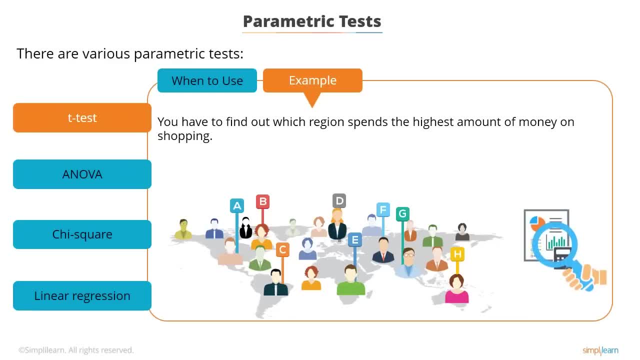 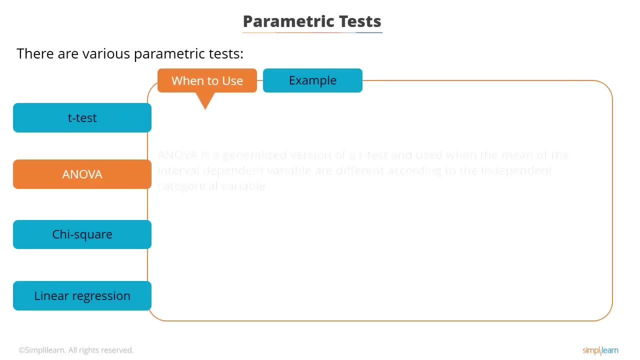 In this example. In this case, you can calculate the highest shopping expenditure by collecting sample observations from each region. With the help of the t-test, you can check if the difference between the regions are significant or a statistical fluke. ANOVA. 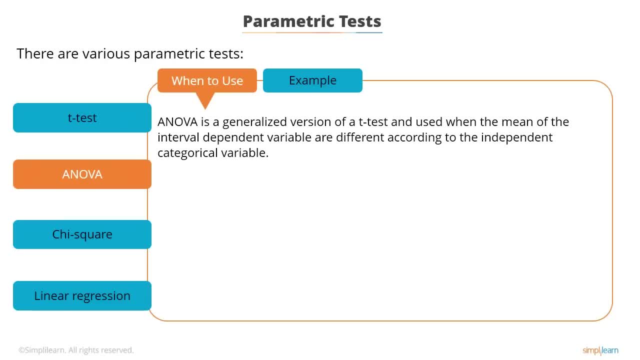 ANOVA is a generalized version of the t-test and used when the mean of the interval dependent variable is different to the categorical independent variable. When we want to check variance between two or more groups, we apply the ANOVA test. For example, let's look at the same example of the t-test example. 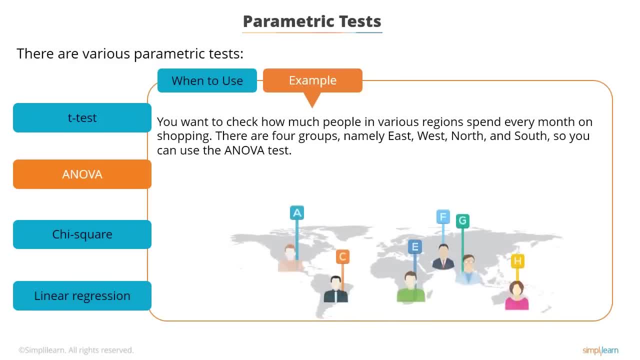 Now you want to check how much people in various regions spend every month on shopping. In this case, there are four groups, namely East, West, North and South. With the help of the ANOVA test, you can check if the difference between the regions is significant or a statistical fluke. 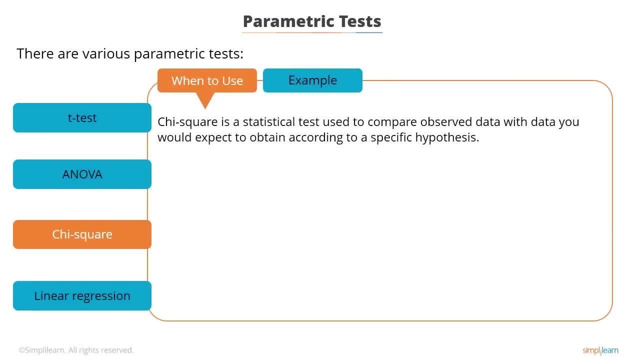 CHI SQUARE. CHI SQUARE is a statistical test used to compare observed data with data you would expect to obtain according to a specific hypothesis. Let's understand the CHI SQUARE test through an example. You have a data set of male shoppers and female shoppers. 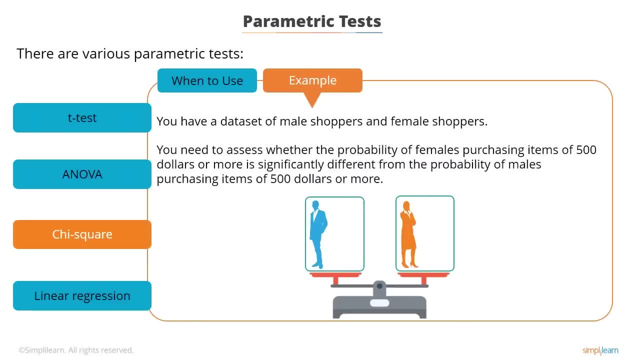 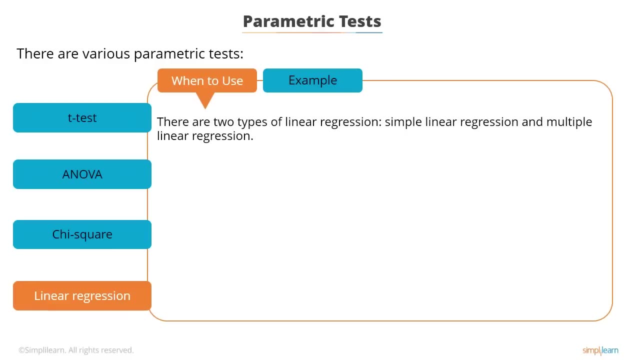 Let's say you need to assess whether the probability of females purchasing items of $500 or more is significantly different from the probability of males purchasing items of $500 or more. LINEAR REGRESSION: There are two types of linear regression: simple linear regression and multiple linear regression. 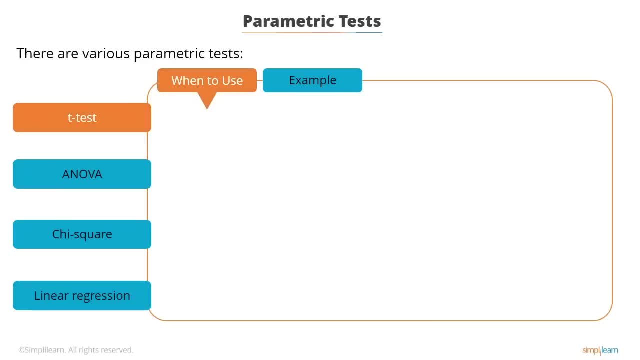 Let's understand them in detail. t-test: A t-test determines if two sets of data are significantly different from each other. The t-test is used in the following situations: To test if the mean is significantly different than a hypothesized value. To test if the mean for two independent groups. 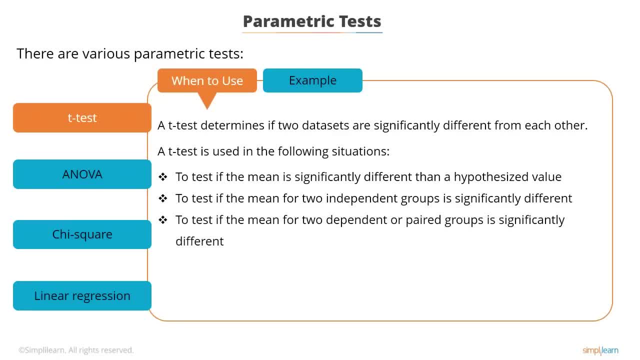 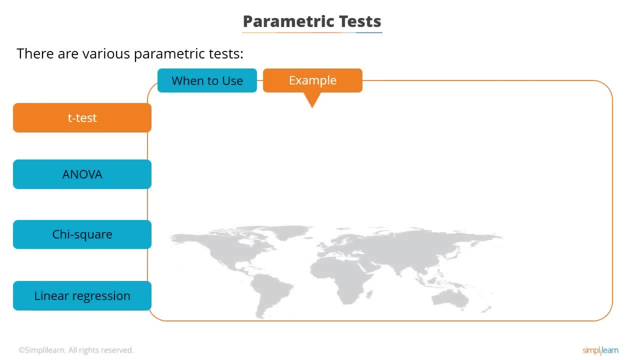 is significantly different. To test if the mean for two dependent or paired groups is significantly different. For example, let's say you have to find out which region spends the highest amount of money on shopping. It's impractical to ask everyone in the different regions. 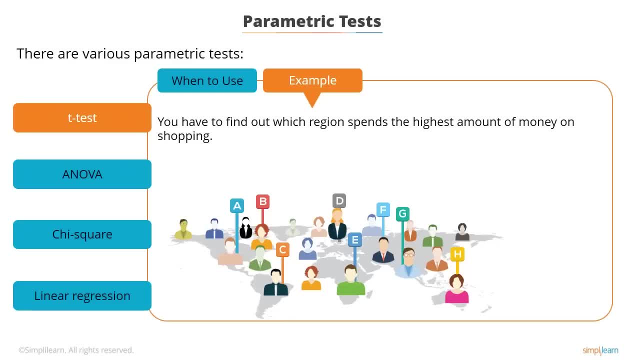 about their shopping expenditure. In this case, you can calculate the highest shopping expenditure by collecting sample observations from each region. With the help of the t-test, you can check if the difference between the regions are significant or a statistical fluke. ANOVA. 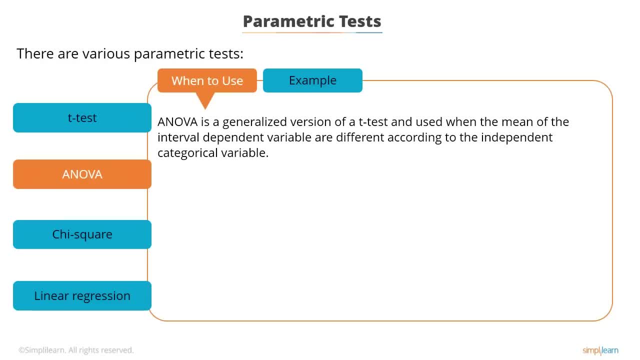 ANOVA is a generalized version of the t-test And used when the mean of the interval dependent variable is different to the categorical independent variable. When we want to check variance between two or more groups, we apply the ANOVA test, For example. let's look at the same example. 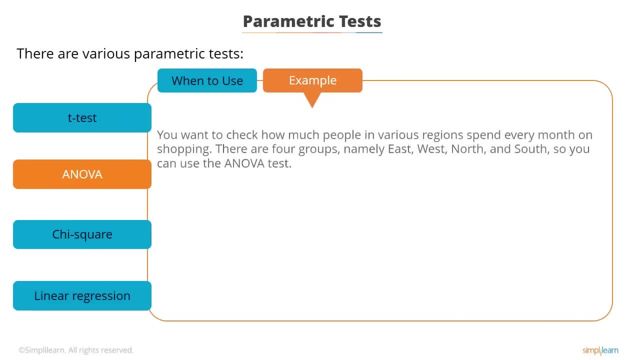 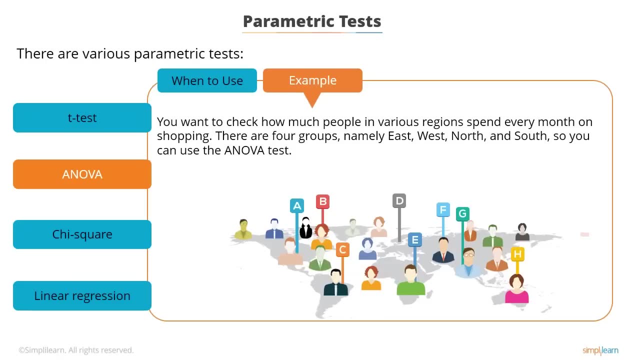 of the t-test example. Now you want to check how much people in various regions spend every month on shopping- In this case, there are four groups, namely East, West, North and South- With the help of the ANOVA test, 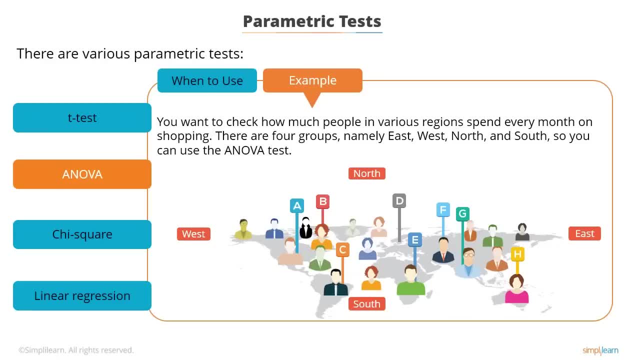 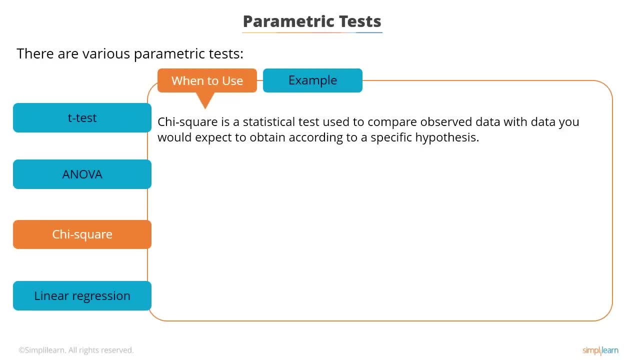 you can check if the difference between the regions is significant or a statistical fluke. CHI-SQUARE. CHI-SQUARE is a statistical test used to compare observed data with data you would expect to obtain according to a specific hypothesis. Let's understand the CHI-SQUARE test through an example. 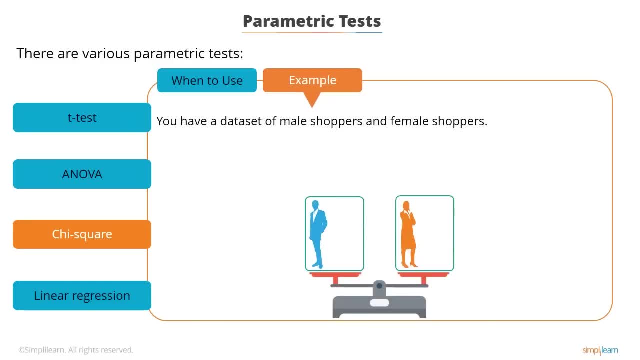 You have a data set of male shoppers and female shoppers. Let's say you need to assess whether the probability of female shopping items of $500 or more is significantly different from the probability of males purchasing items of $500 or more. LINEAR REGRESSION. 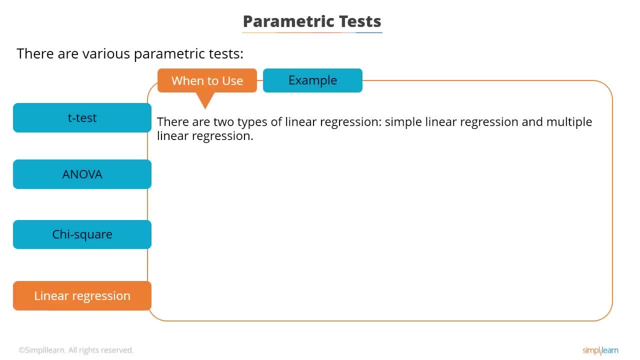 There are two types of linear regression: simple linear regression and multiple linear regression. Simple linear regression is used when one wants to test how well a variable predicts another variable. Multiple linear regression allows one to test how well multiple variables or independent variables predict a variable of interest. 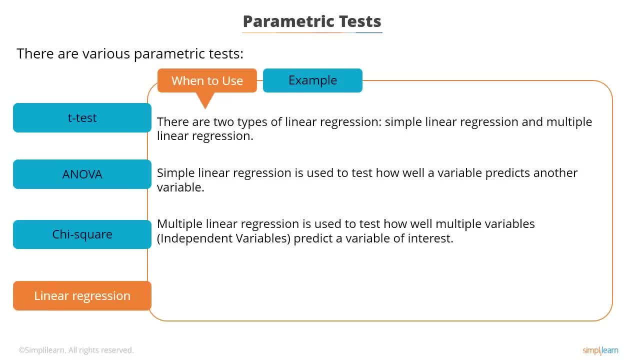 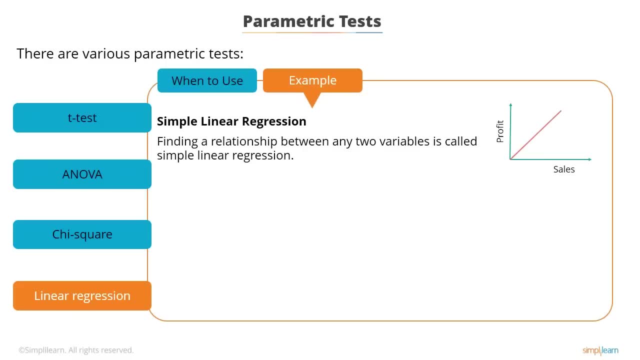 When using multiple linear regression, we additionally assume the predictor variables are independent. For example, finding relationship between any two variables, say sales and profit, is called simple linear regression. Finding relationship between any three variables, say sales, cost and telemarketing. 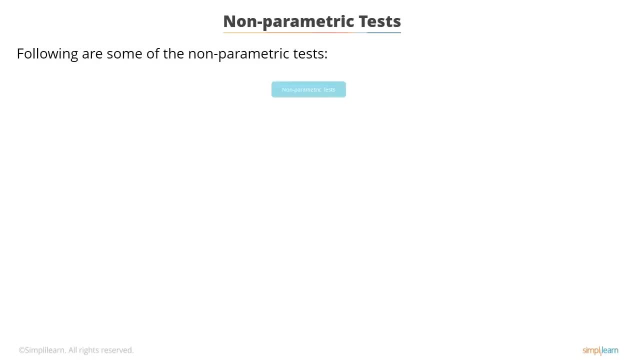 is called multiple linear regression. Some of the non-parametric tests are Wilcoxon rank sum test and Kruskal-Wallis H-test. Wilcoxon rank sum test- The Wilcoxon signed rank test- is a non-parametric statistical hypothesis test. 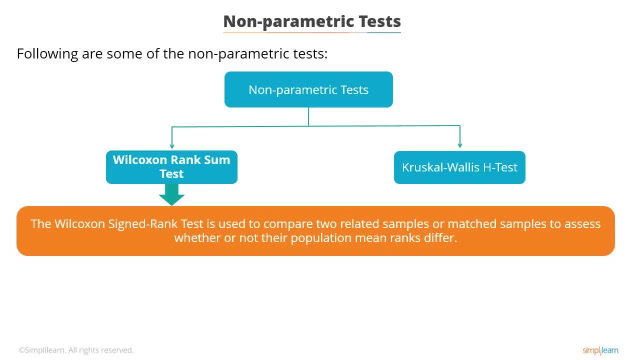 used to compare two related samples or matched samples to assess whether or not their population mean ranks differ. In Wilcoxon rank sum test you can test the null hypothesis on the basis of the ranks of the observations. Kruskal-Wallis H-test. 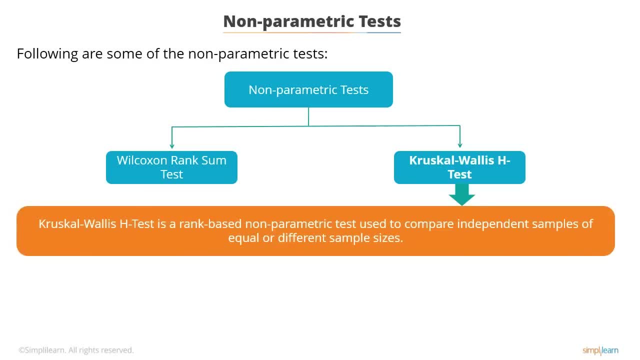 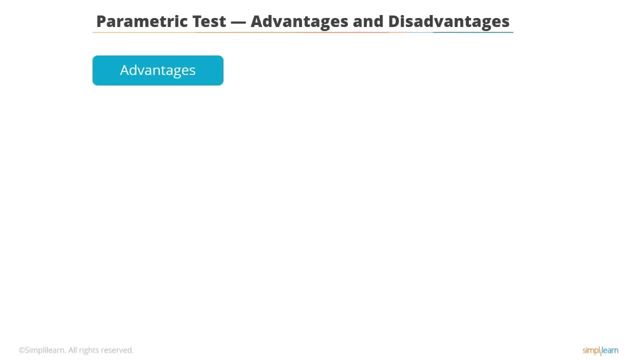 Kruskal-Wallis H-test is a rank-based non-parametric test used to compare independent samples of equal or different sample sizes. In this test, you can test the null hypothesis on the basis of the ranks of the independent samples. The advantages of parametric tests. 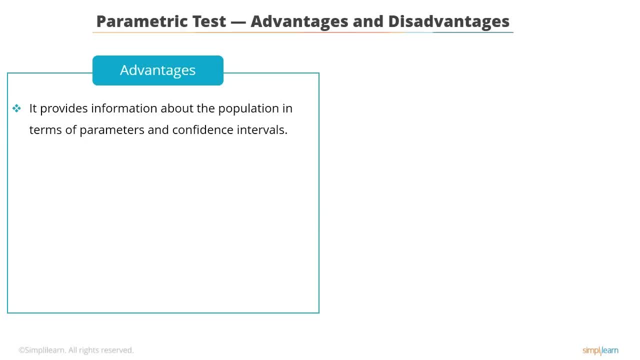 are as follows: Provide information about the population in terms of parameters and confidence intervals, Easier to use in modeling, analyzing and for describing data potential tendencies and data transformations. Express the relationship between two or more variables. Don't need to convert data. 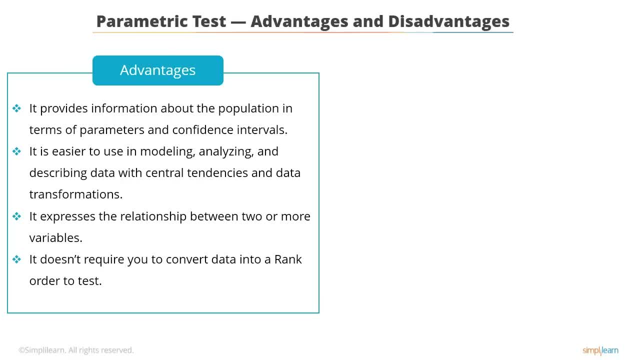 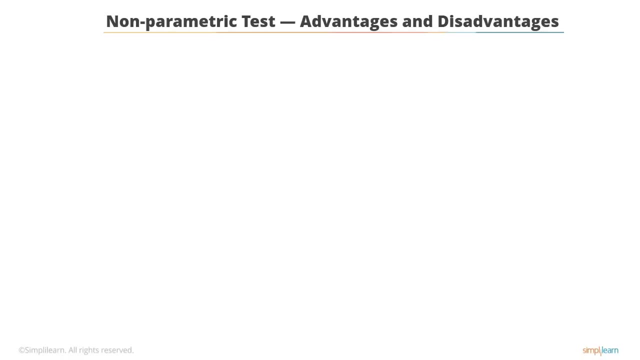 into rank order to test. The disadvantages of parametric tests are as follows: Only support normally distributed data. Only applicable on variables, not attributes. Let's now list the advantages and disadvantages of non-parametric tests. The advantages of non-parametric tests. 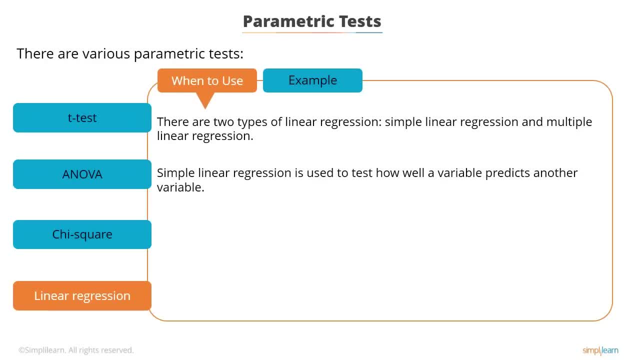 Simple linear regression is used when one wants to test how well a variable predicts another variable. Multiple linear regression allows one to test how well multiple variables or independent variables predict a variable of interest. When using multiple linear regression, we additionally assume the predictor variables. 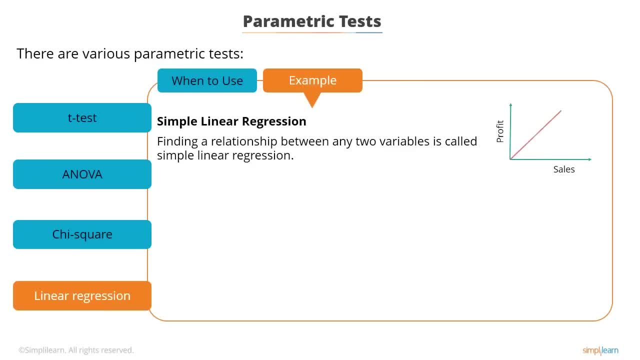 and the predictor variables are independent. For example, finding relationship between any two variables, say sales and profit, is called simple linear regression. Finding relationship between any three variables, say sales, cost and telemarketing, is called multiple linear regression. 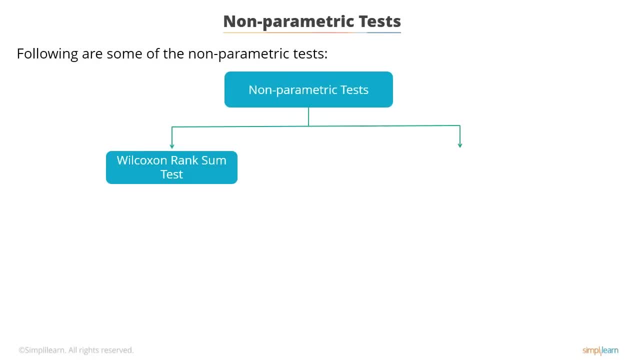 Some of the nonparametric tests are Wilcoxon Rank Sum Test and Kruskal-Wallis H Test. Wilcoxon Rank Sum Test: The Wilcoxon Signed Rank Test is a nonparametric statistical hypothesis test used to compare two related samples or matched samples. 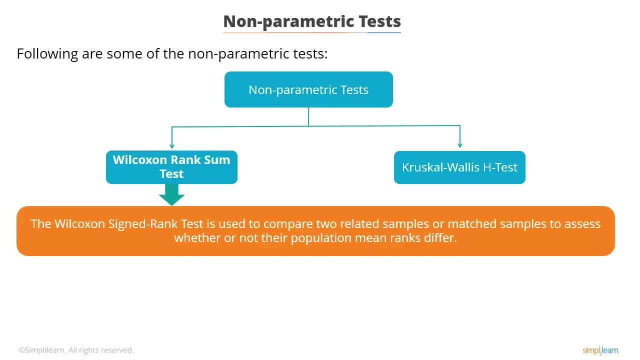 to assess whether or not their population mean ranks differ. In Wilcoxon Rank Sum Test, you can test the null hypothesis on the basis of the ranks of the observations. Kruskal-Wallis H Test. Kruskal-Wallis H Test is a rank-based nonparametric test used to compare independent samples of equal or different sample sizes. 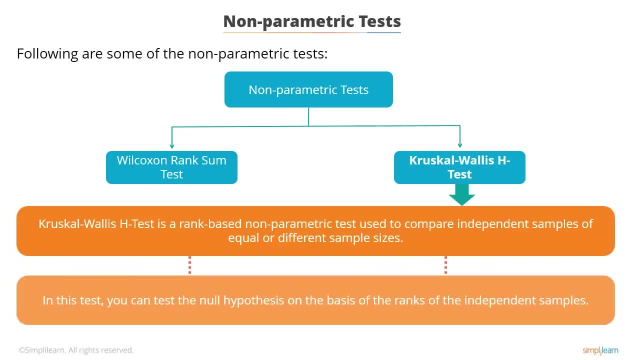 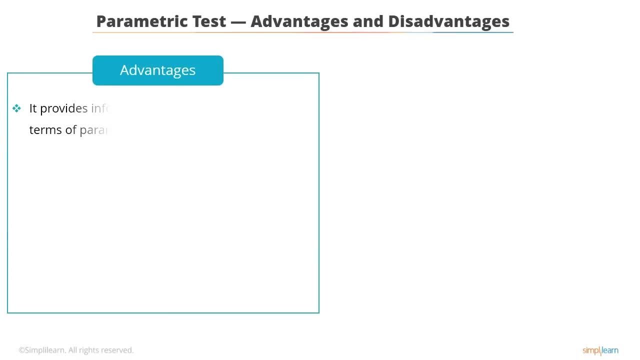 In this test, you can test the null hypothesis on the basis of the ranks of the independent samples. The advantages of parametric tests are as follows: Provide information about the population in terms of parameters and confidence intervals Easier to use in modeling, analyzing and for describing data with central tendencies and data transformations. 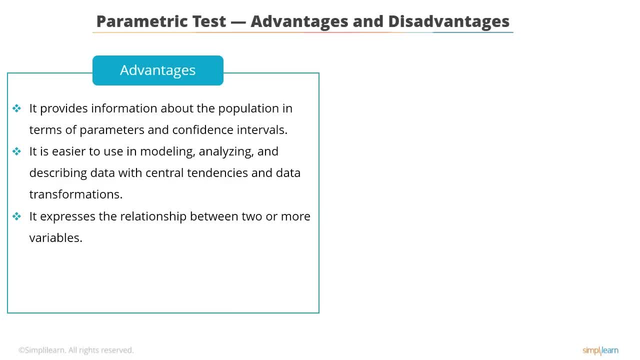 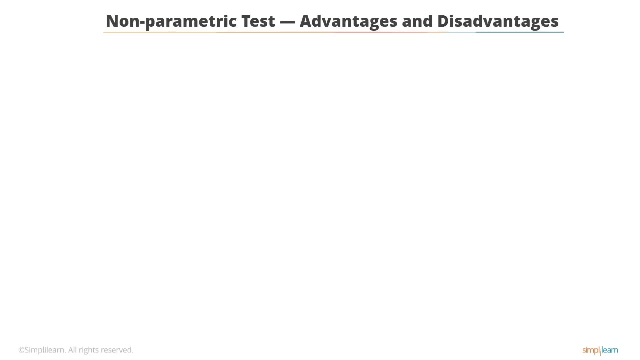 Express the relationship between two or more variables. Don't need to convert data into rank order to test. The disadvantages of parametric tests are as follows: Only support normally distributed data. Only applicable on variables, not attributes. Let's now list the advantages and disadvantages of nonparametric tests.